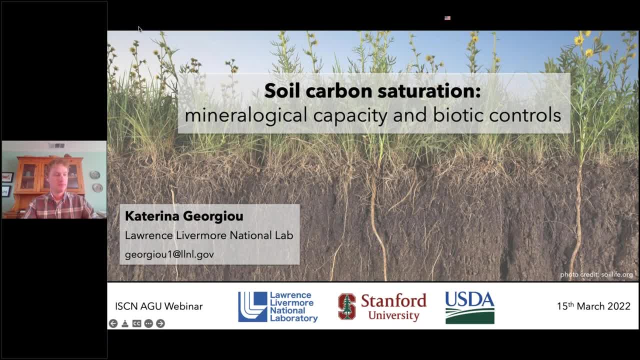 All right, well, I'd like to roll into our first talk, but one last thing before I do is to remember that you can post questions via the questions feature and then I will relay them to the speakers. We'll have two Q&A sessions, one after each talk. Thank you, 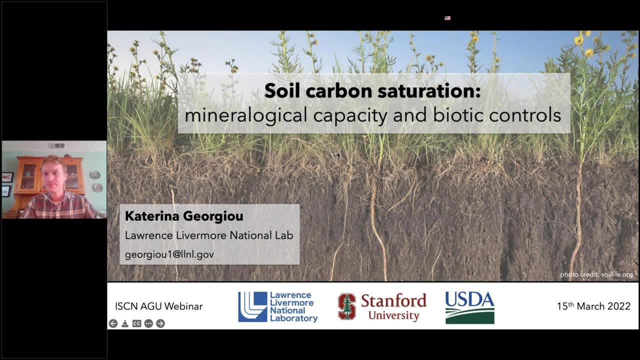 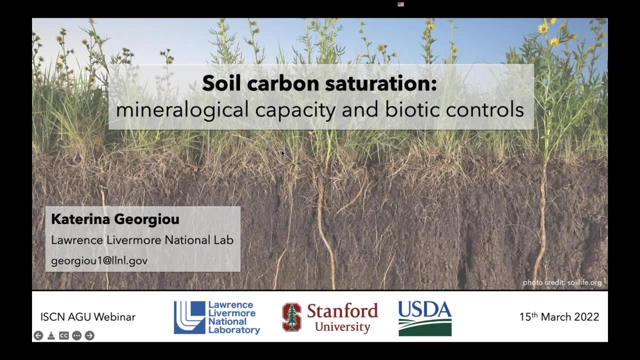 very much. And, Kat, why don't you take it from here? Great Thanks, Eric, And I apologize. my video. I have technical difficulties so we weren't able to sort it out, But I'm really excited to speak to you all today about soil carbon. 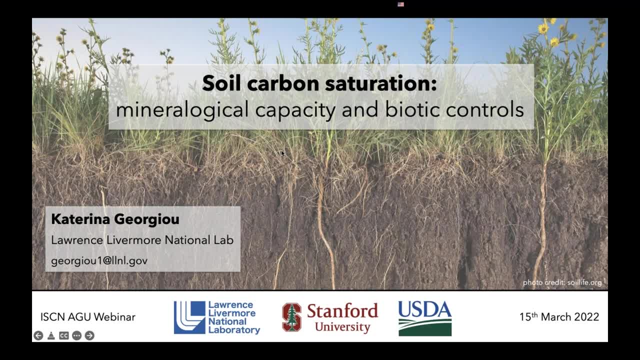 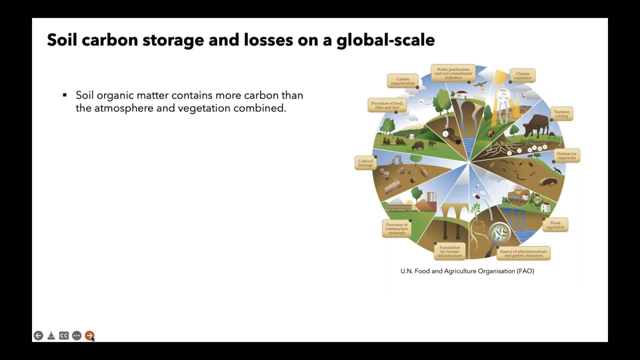 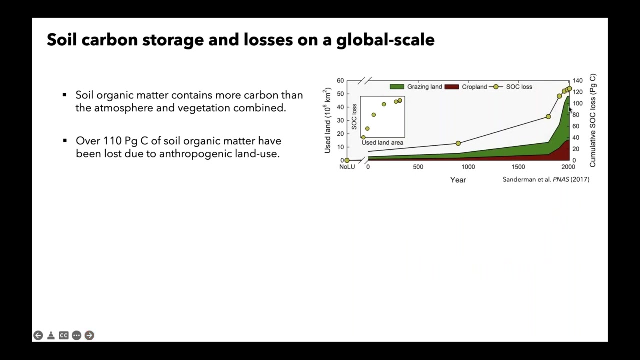 saturation, both mineralogical capacity and biotic controls. So soil organic matter is, of course, an enormous pool of carbon globally and has many other important ecosystem functions, And over the course of history about 110 petagrams of carbon have been lost from soils due to human land use. 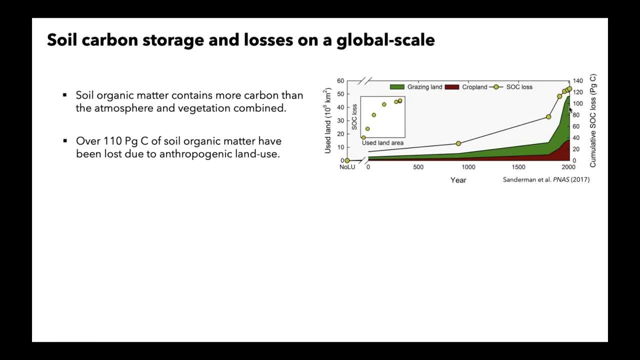 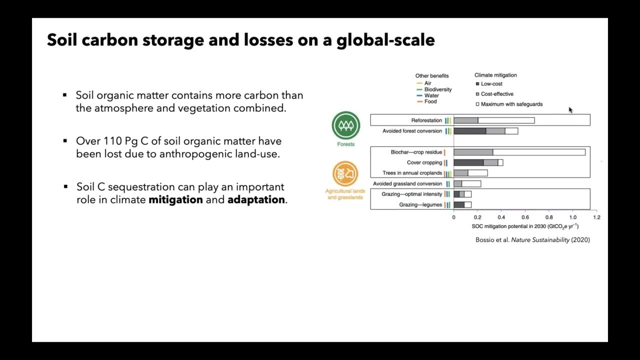 This soil carbon debt suggests that there could be potential for targeted soil. targeted carbon accrual in soils And such soil carbon sequestration practices can play an important role in climate mitigation, as shown in this diagram, but also an adaptation with many co-benefits for food, water and biodiversity. But as we talk about soil carbon sequestration, 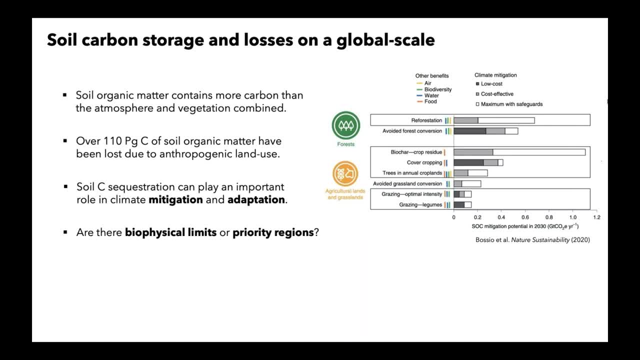 it's important to consider whether there are biophysical limits or priority regions. So today I'd like to talk about two key functional pools in soils and how their dynamics differ, especially with regards to saturation. I'll introduce the concept of soil carbon saturation and some common misconceptions. I'll present results from a key study at a global scale. 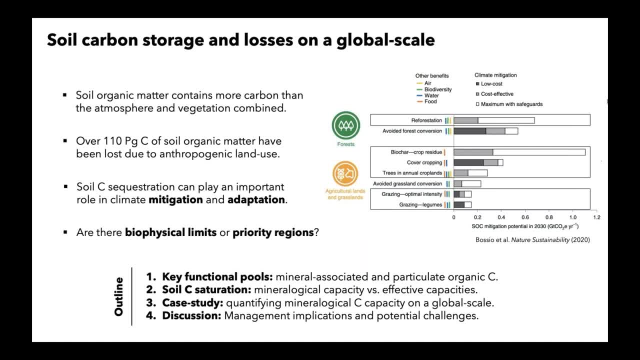 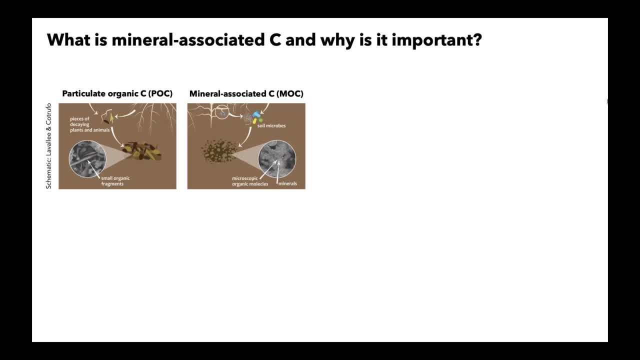 quantifying mineralogical limits and finally end with some management implications and potential challenges. So first, two key functional pools in soil are mineral associated carbon and particulate organic carbon. And mineral associated carbon is composed of organic matter that's often microbially processed and is bound or absorbed to mineral surfaces. 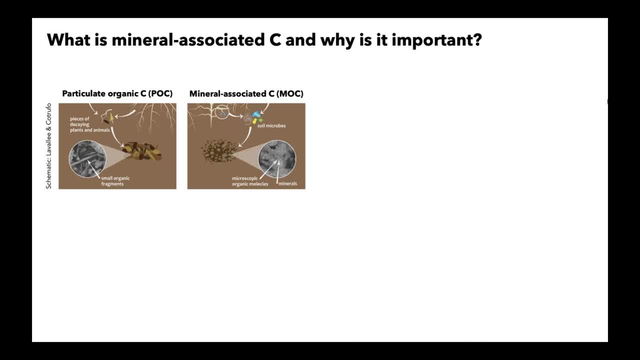 In contrast, particulate organic carbon is often small organic fragments that are not associated with mineral particles. And this mineral associated carbon pool, which we'll largely focus on today, is important because it constitutes the majority of soil carbon. It's also important because it's the largest carbon in mineral soils globally, but also 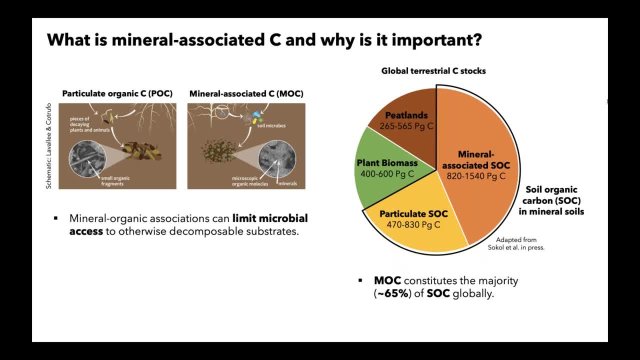 because these mineral organic associations can limit microbial access to otherwise decomposable substrates And so, as a result, mineral associated carbon can be much older than particulate carbon at the same depth, And because of this, mineral associated carbon could be important for lasting carbon storage in soils. But mineral surfaces may have a finite capacity that can 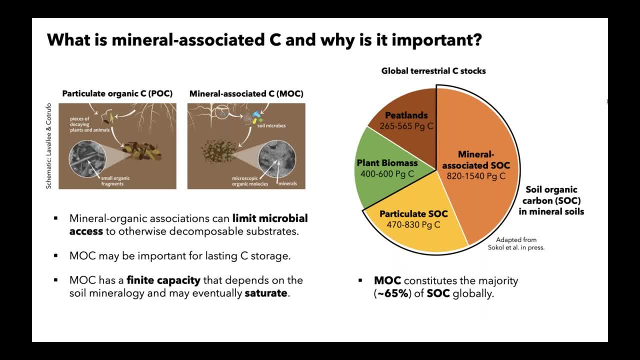 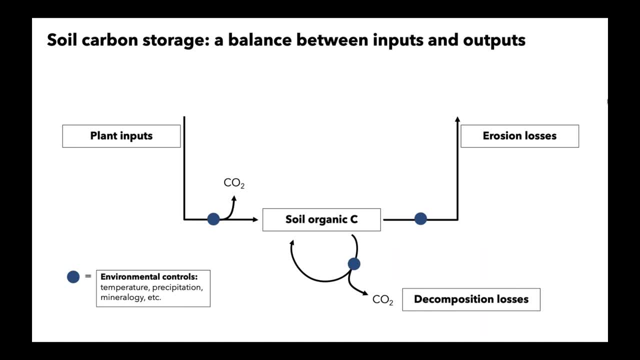 depend on the soil mineralogy that may eventually saturate. So, before we dive into soil carbon saturation, I'd like to revisit the fact that soil carbon storage is a balance between inputs and outputs, where the various transformations can additionally be controlled by a number of environmental factors. And so, to increase soil carbon, we 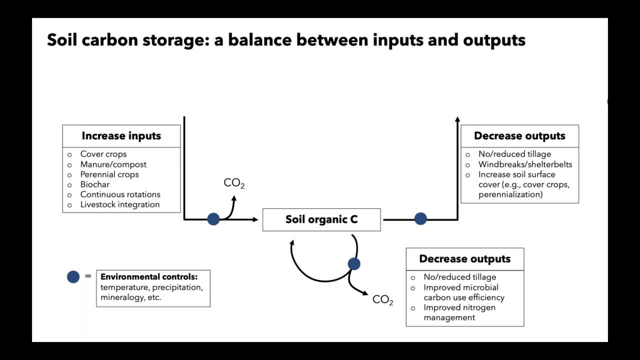 can either increase inputs, for example with cover crops or soil amendments, or we can decrease outputs, for example using windbreaks or shelterbelts to reduce wind pressure, And by doing so we can extend soil carbon to a number of different sounds. Bye. 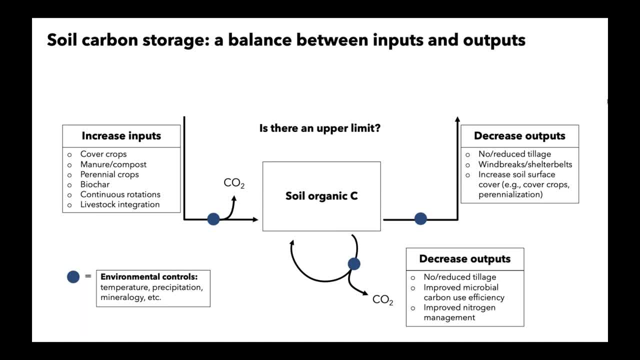 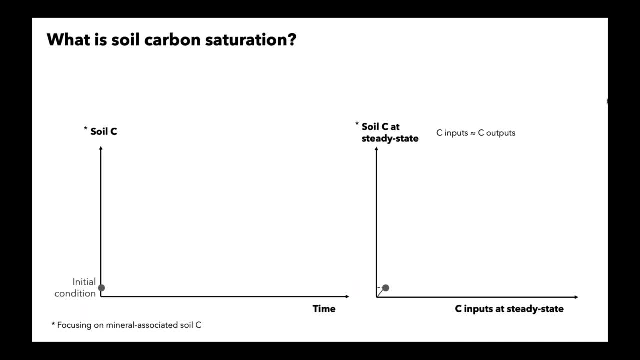 Toby, did you have a question on soil carbon? Yeah, Oh, um, yeah, Um, I think so And I'm sorry. I think that's a great answer And that's a really good answer, but I do have to say that soil carbon is not always. 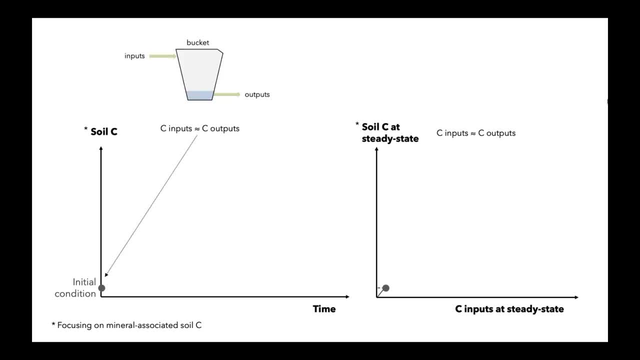 the most effective tool when looking at soil carbon Right. So soil carbon's really important. Right this example, I'll have a bucket analogy where we'll be filling a bucket of water as sort of a total mineralogical capacity, as an analogy for the mineralogical capacity. so, starting from some 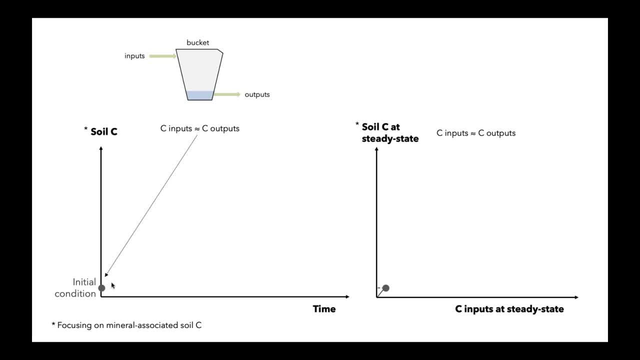 initial conditions, say a degraded soil that has low soil carbon and carbon inputs at steady state, where carbon inputs are equal to outputs. we could potentially increase soil carbon by increasing inputs, for example with cover crops or soil amendments, and at this point carbon inputs could be greater than carbon output. so we can see an increase in soil carbon over time. on the left: 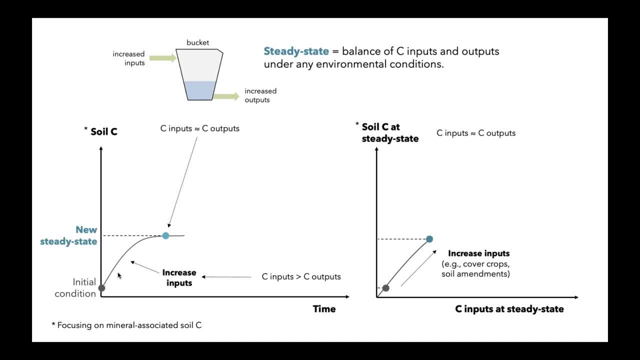 panel up till some steady state where the carbon outputs catch up with the carbon inputs. and I'd like to note here that just because the soil has received carbon inputs for a long time does not indicate saturation. in fact, it could just indicate that it's at a steady state. 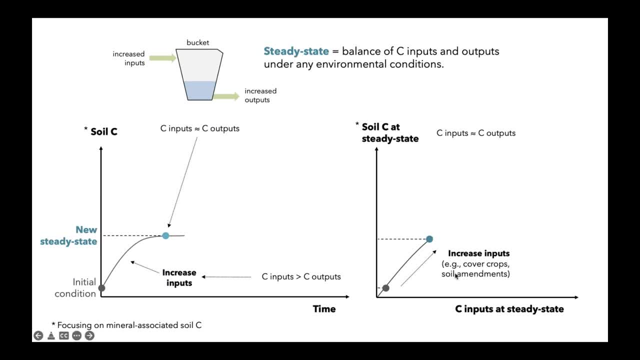 and so we can see on the right panel that further increasing inputs could lead to further increase in soil carbon up to some new steady state, which here we can see a plateau in the relationship between soil carbon and carbon inputs, and so this is a resembles a saturation. 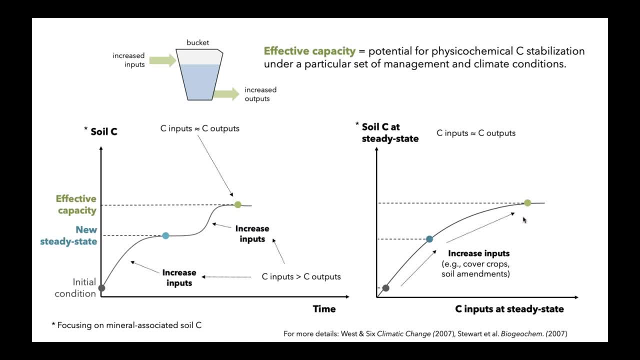 but this could be limited to the particular set of management and climate conditions of a certain soil. and theBut this could be limited to the particular set of management and climate conditions of a certain soil. and carbon the soil, For example, if the soil was under tillage, decreasing tillage to decrease outputs. 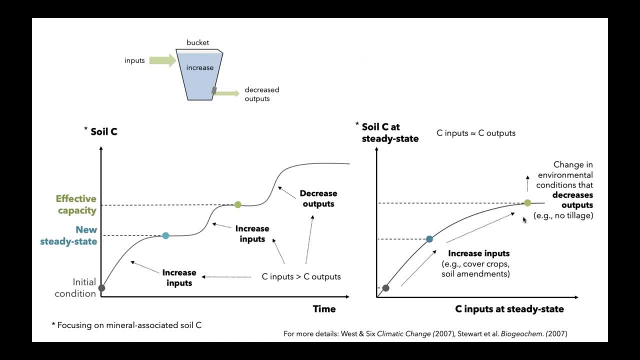 could lead to a further increase in soil carbon up to some new steady state, potentially mineral saturation. And so the saturation we'll define here as a theoretical maximum capacity, mineralogical capacity under optimum conditions, So independent of management and climate, And this 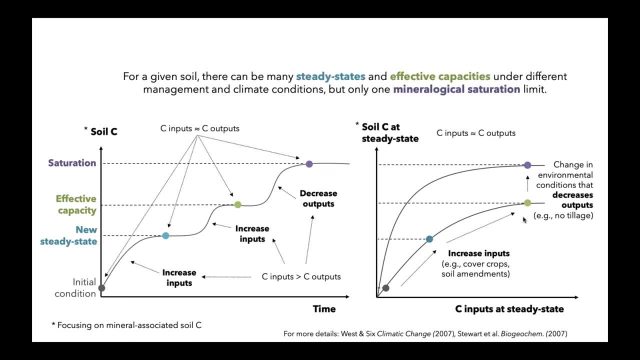 is important to keep in mind. So for a given soil, there can be many steady states and effective capacities under different management and climate conditions, but only one mineralogical saturation limit. And this saturation limit can be unique to a given soil based on its mineralogy. 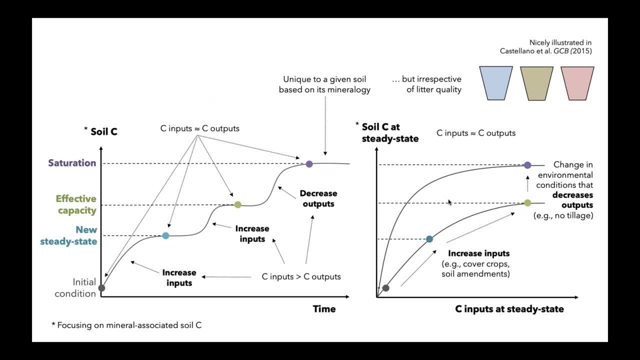 or the size of the bucket. But while litter quality can control the proximity or the approach of a soil towards saturation, the mineralogical limit itself is independent of the litter quality, And this is nicely illustrated in this paper by Castellano et al in 2015.. 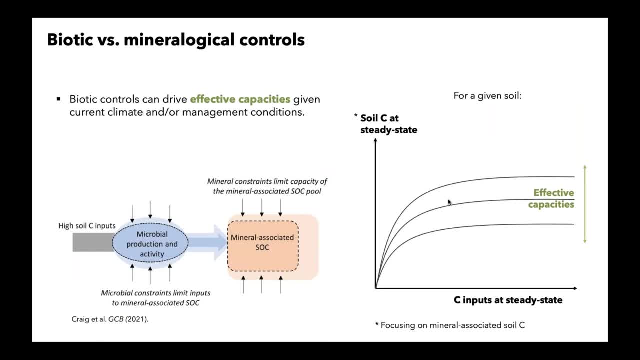 So these effective capacities can be can be driven by biotic controls, given the current climate and or management conditions- And this is nicely illustrated in this paper by Matt Craig and colleagues- where even for a high increase in soil carbon inputs, there could be microbial constraints. 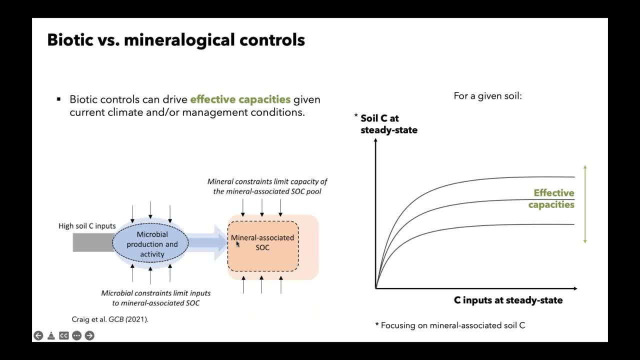 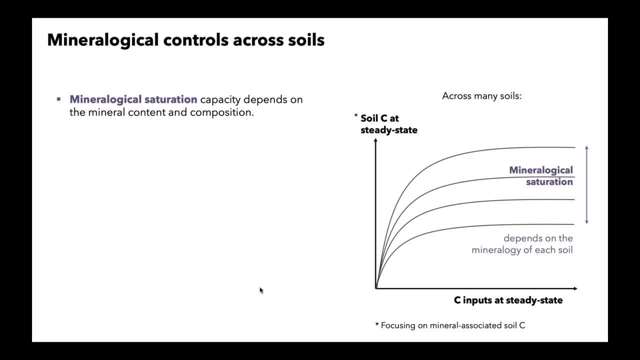 That limit inputs into the mineral associated carbon pool So that it's difficult to achieve the full mineralogical saturation which be indicated by this larger orange box here When we look across many soils. the mineralogical saturation can depend on the mineral content and 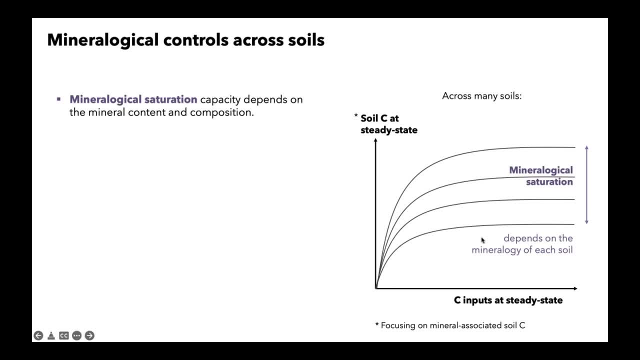 composition And so we might have many curves across many soils. So it can be difficult to quantify or even observe mineralogical saturation In this way across many soils with different climate and management conditions. For example, in the synthesis by Stuart at all with soil carbon versus carbon input across 14,. 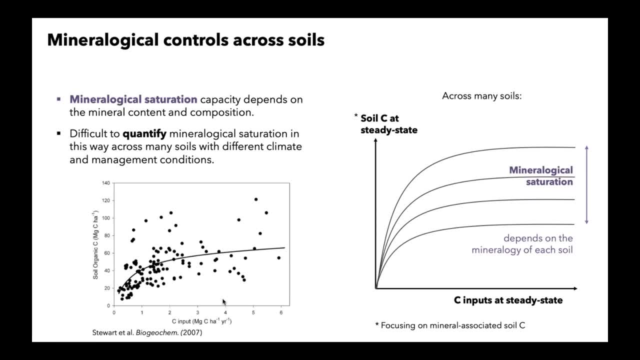 long term manipulation experiments. we could in fact have not just one saturation curve but many, depending on the soil mineralogy. But as I mentioned earlier, we would not get 100% of the soil after the primer. So we would actually get 1% of the soil after the primer, but we would still have at least 10% of the soil. 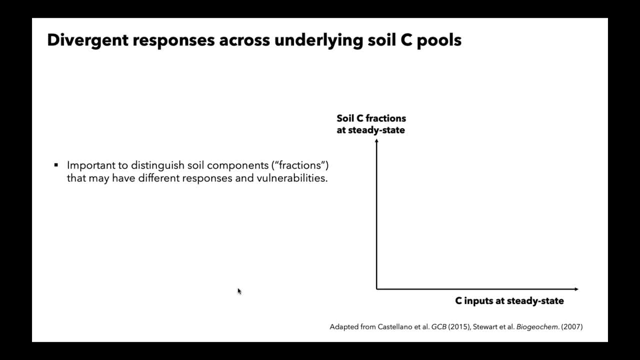 But, as I mentioned earlier, we would not get 100% of the soil after the primer mentioned earlier. it's also important to note that there can be different soil components or fractions that have different responses and vulnerabilities. For example, mineral-associated carbon, which we've been conceptually focusing on so far, which is expected to saturate. 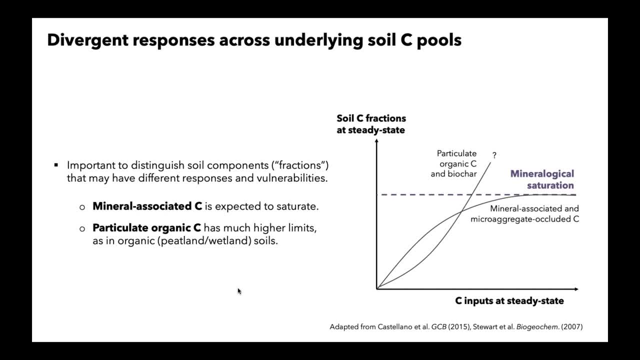 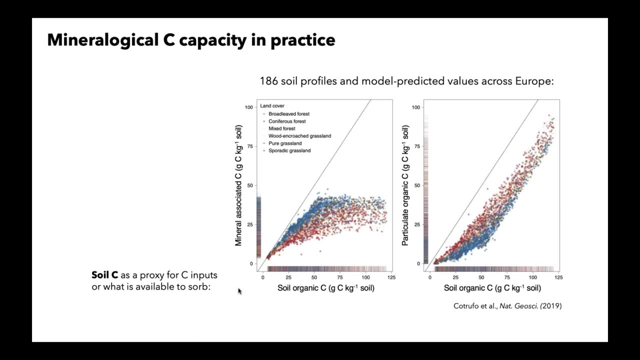 but also particulate organic carbon, which can have much higher limits, as seen in organic peatland or wetland soils, And these divergent dynamics between these pools were nicely illustrated in a recent paper by Francesco Petruppo and colleagues, where they use 186. 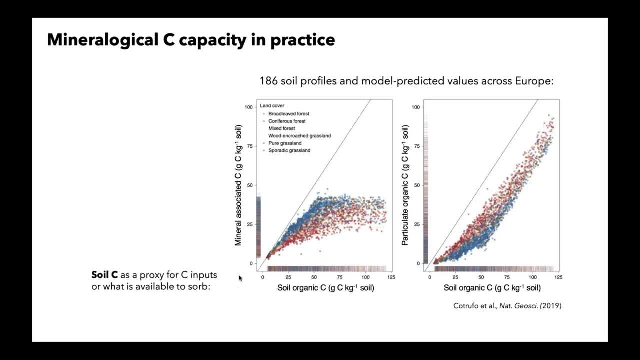 soil profiles and model predicted values across Europe to explore the relationship of mineral-associated carbon and particulate organic carbon as a function of total soil, organic carbon as a proxy for carbon inputs or what's available to XOR. And so indeed we can see this saturating behavior of the mineral-associated pool and 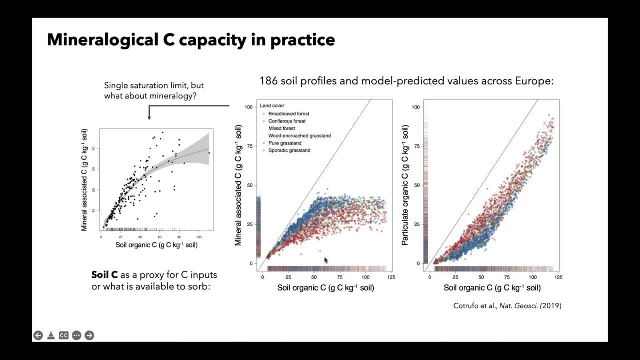 an increase in the particulate pool. So we might be tempted to fit a saturation curve to these soil profiles to determine saturation limit. but as we discussed before, the saturation limit can critically depend on the mineralogy. So we could imagine that a soil with very low clay content has a different mineralogical. 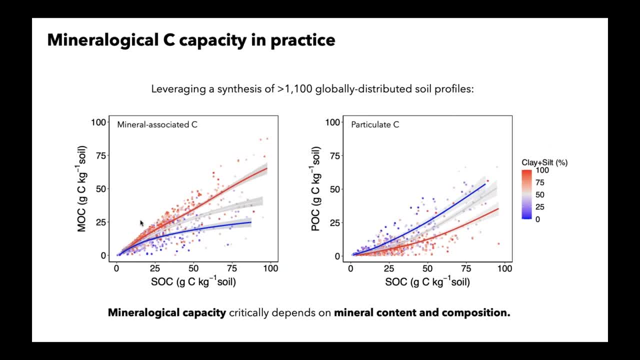 limit than a soil with very high clay content. And so we can see just that when we look across a synthesis of 1100 soil profiles around the globe. And we have the same figures here: mineral-associated carbon and particulate organic carbon, but now colored by clay and silt content. 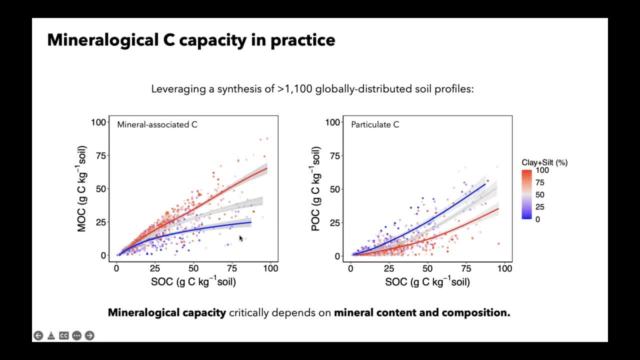 And we can see that the asymptote of these saturation curves can critically depend on the mineral content which I'm showing here, but also the composition, which I'll come back to later. So it can be very difficult to fit the mineralogical limit in this way across many different soils. And so how was this mana- how's this? 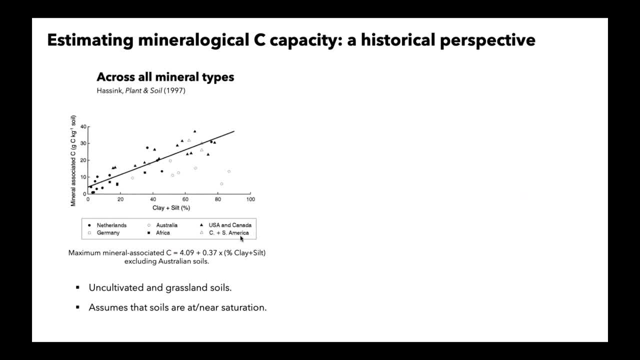 mineralogical capacity fit in practice. So in this seminal work by Hann Höh記, because of this importance of clay and silt content, we can explore the relationship between mineral-associated carbon, carbon in clay and silt, And in this work, by Async, uncultivated and grassland soils that 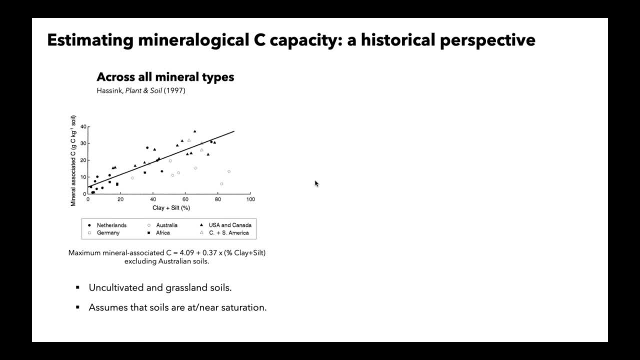 were assumed to be at or near saturation were used, with a linear regression, to estimate this potential limit at saturation. But, as we mentioned earlier, just because a soil has received inputs for a long time and is at some steady state, it's still no indication that the soil is at saturation. 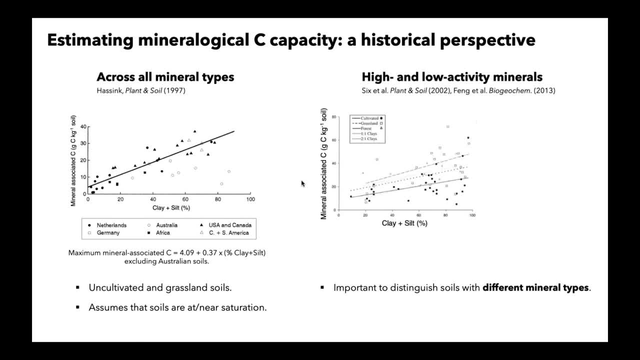 Further work by Johan Six and colleagues explored introducing different mineral types, which we'll come back to later, because of different reactive surface areas between minerals, And Wenting Feng and colleagues also argue that their boundary lines are more appropriate than a linear regression for fitting a maximum mineralogical capacity. 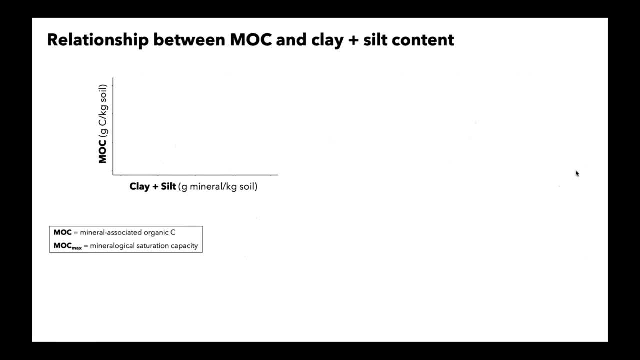 So to understand why that is, let's first take a look at what this relationship implies. So, with mineral-associated carbon on the y-axis and clay and silt on the x-axis, the slope here denotes some grams carbon per gram mineral, And of course we don't expect this to be a universal value. 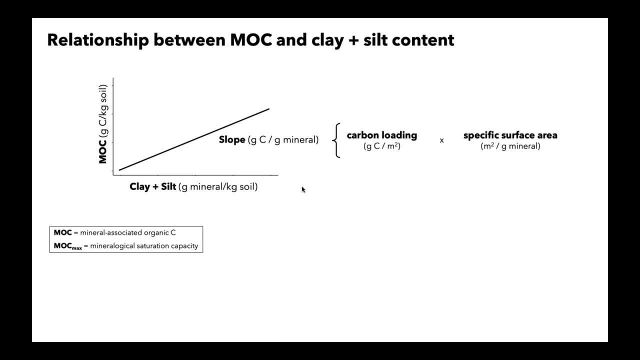 because it can depend on the carbon loading and the specific surface area, Where the surface area is the carbon loading and the specific surface area. Where the surface area is the carbon loading and the specific surface area can depend on the mineral type. For example, when 1 to 1 and 2 to 1 phyllosilicate clays that can have low and high reactive surface. 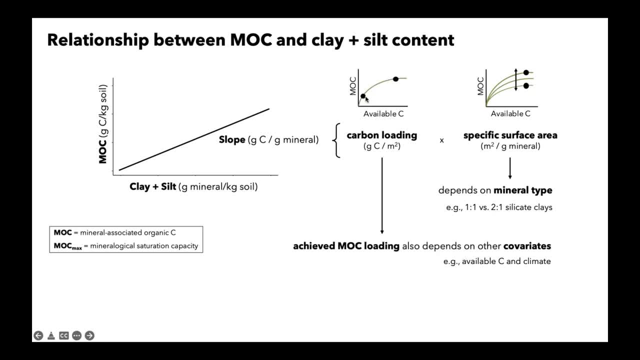 areas respectively, but also the carbon loading, or how full the bucket is. the achieved carbon loading can depend on a number of other covariates, including climate and management, And so at a maximum carbon loading at the mineralogical capacity, we expect this capacity to be largely a function of the mineral content and composition. 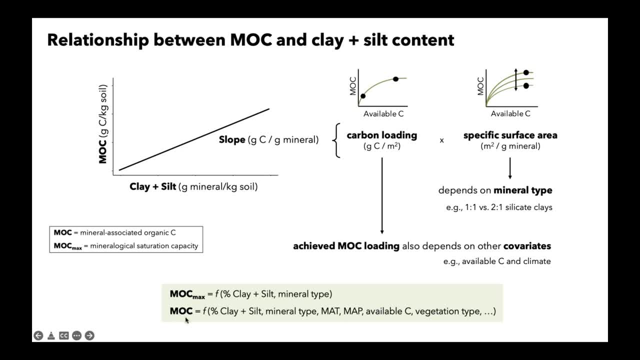 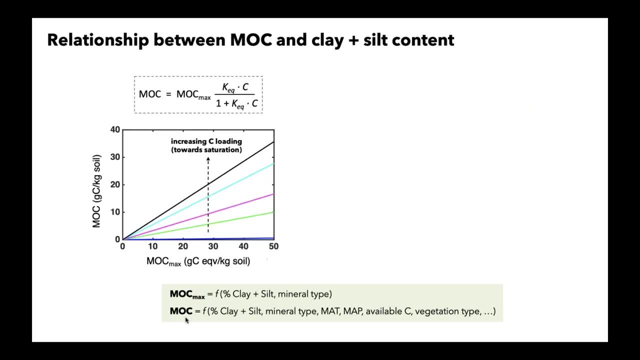 but the achieved mineral-associated carbon can also depend on a number of other climate and management factors And soil. biogeochemical models also suggest this behavior, where, with increasing carbon loading, we have increasing slopes up till some saturation, And so, instead of a linear regression, fitting a maximum slope can give us an estimate of the. 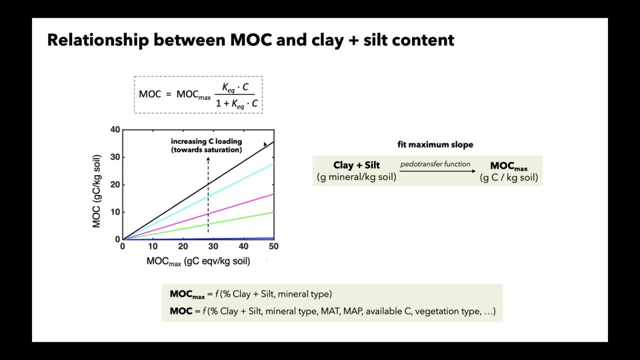 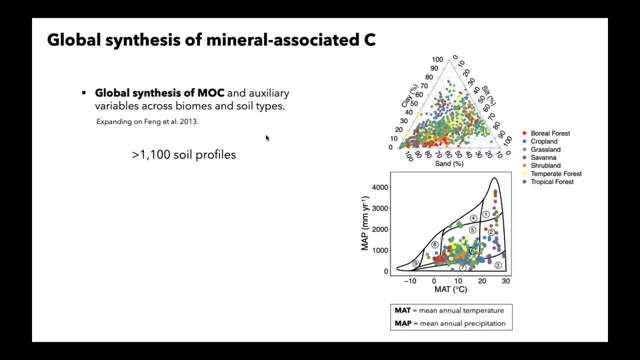 mineralogical capacity, assuming that there's enough variability globally that this capacity is reached. And so, in order to constrain this at the global scale, we conducted a synthesis of mineral الص Figure carbon across 1,100 soil profiles, where here you can see the clay, silt and sand. 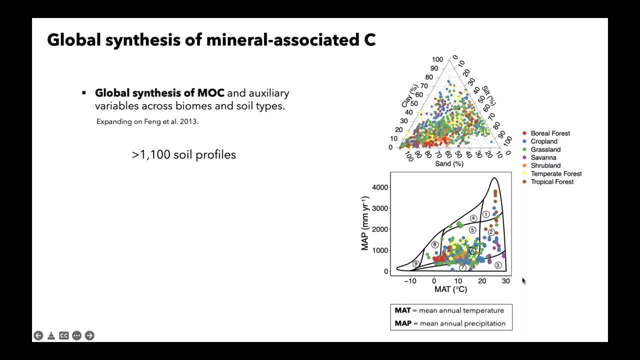 content across the profiles, the mean annual precipitation versus temperature of the profiles. so they span many biomes and soil types worldwide and we can take a look at this relationship between mineral, associated carbon and clay and silt content across these profiles and so we can already see an envelope begin to. 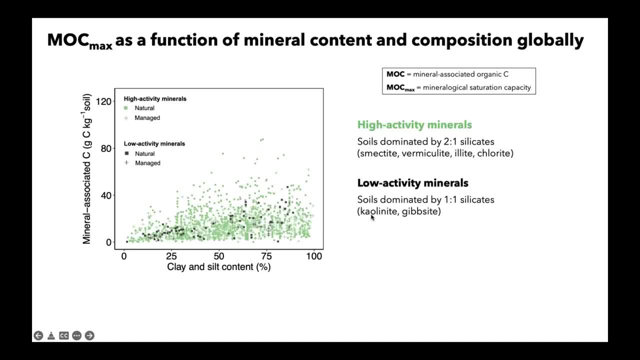 emerge here, and this is even more clear when we separate soils based on their mineral activity, where here we've separated soils into into soils dominated by two to one phyllosilicate as high activity minerals and one-to-one phyllosilicate as low activity minerals. 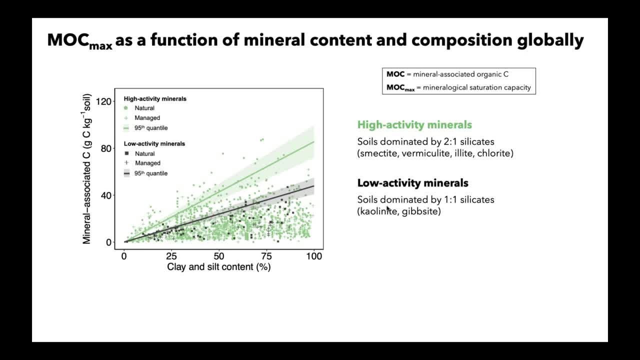 and fitting a conservative boundary line to these points. using a 95th quantile with 90 prediction intervals, we can estimate this mineralogical capacity for across the different mineral types and we can use these functional relationships along with maps of mineral content and carbonation, and so we can see that these are different functional relationships and we can use. 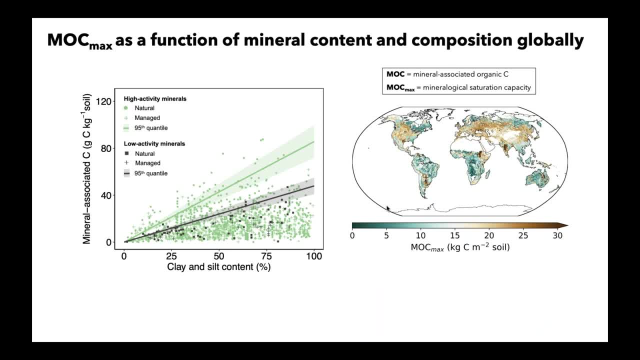 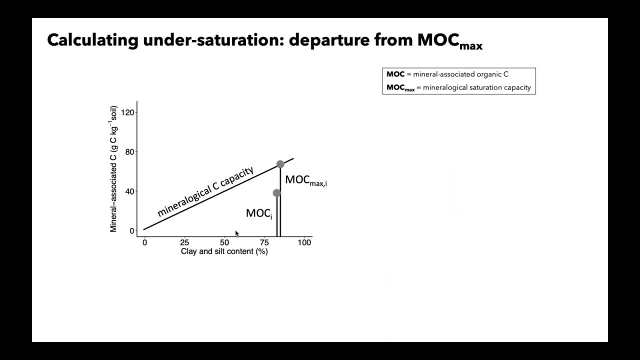 position at a global scale in order to estimate this mineralogical capacity across soils globally. But, as you can see, there are many points below this mineralogical capacity. and so what drive, what factors drive this observed variability, And so, to explore this, we can calculate the percent saturation or the proximity of a soil. 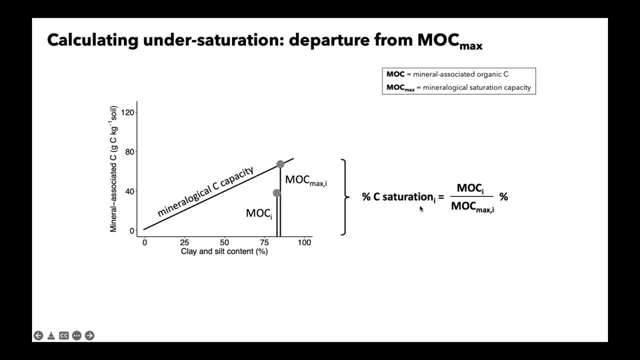 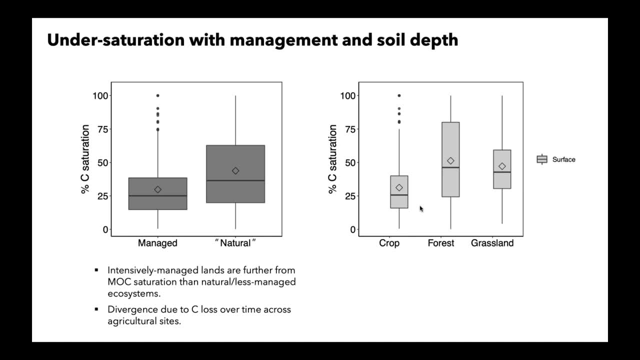 to its mineralogical capacity and we expect this percent saturation to be a function of management as well as depth and climate. So first, broadly grouping soils in terms of management, we can see that intensively managed agricultural lands tend to be further from mineralogical saturation than natural or less managed. 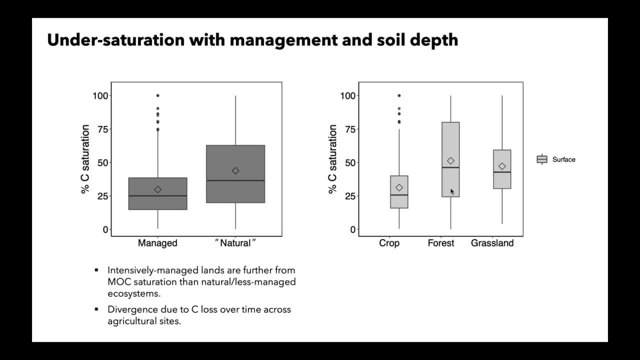 grassland and forest ecosystems, and this divergence is likely due to carbon losses over time across the agriculture. We can also see that deeper soil layers tend to be further from saturation than surface soil layers, likely due to lower inputs at depth, but interestingly we find that grasslands are closer to mineralogical saturation at depth than other ecosystems. 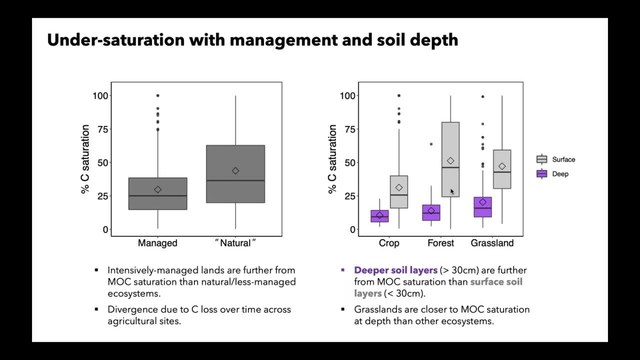 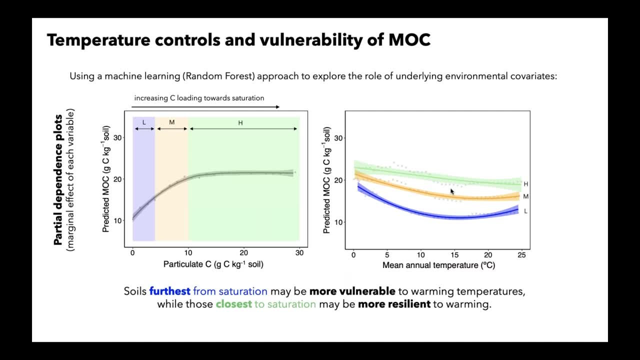 potentially due to their extensive and deep rooting systems. We also used a machine learning, a random forest approach, to explore the role of underlying environmental covariance, And so here I'm showing partial dependence plots that depict mineral associated carbon as a function of each variable, controlling for all other variables and in this case particulate organic. 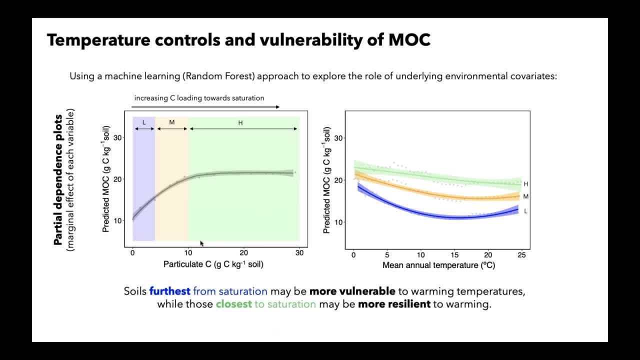 carbon as a proxy for what is available to Zorb and we can see an increase in mineral associated carbon with increasing carbon loading up to some carbon saturation and also as a function of mean annual temperature. In general, we see that mineral associated carbon decreases as a function of increasing temperature. 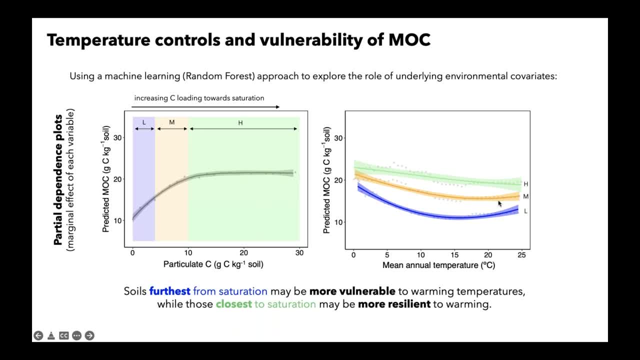 but interestingly we find that this this behavior differs depending on the saturation regime, where soils furthest from saturation may be more vulnerable to warming, while those closest to saturation may be more resilient, and so this has additional implications for for adaptation and resilience. So, using this synthesis, 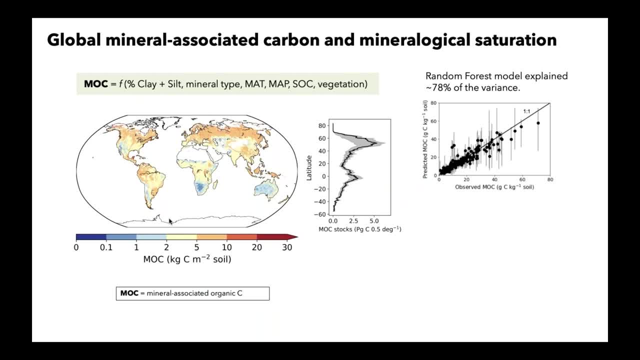 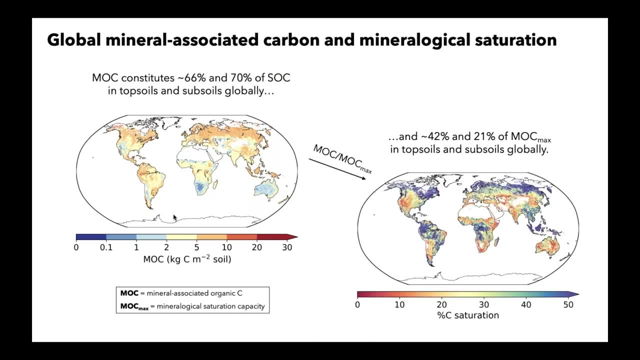 we can also estimate the current mineral associated carbon stocks globally, again using a random forest model with 90 percent prediction intervals, and we can use this with our maps of mineralogical capacity to estimate the percent saturation of soils globally, And so you may wonder if soils are only 20 or 40 percent of their mineralogical. 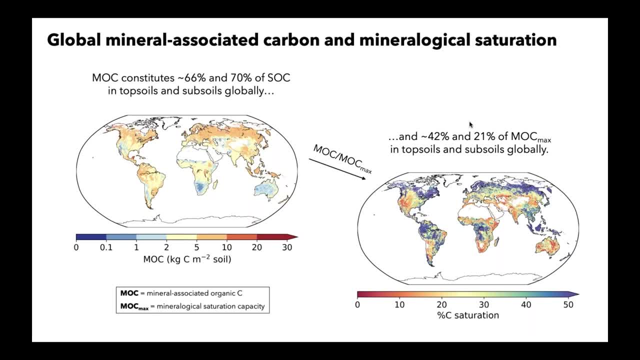 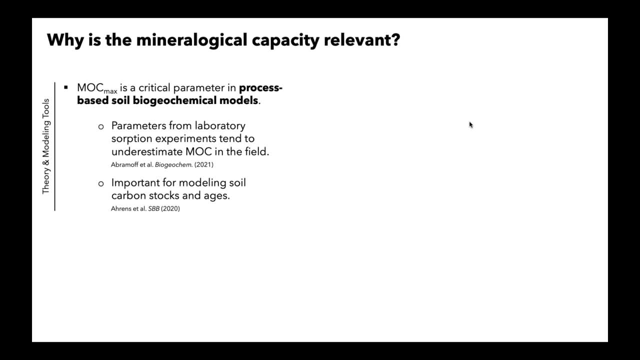 but of the mineralogical saturation. then is this limit really relevant? Well, yes, for several reasons. first, from a theoretical or modeling perspective. it's a critical parameter in process-based soil biogeochemical models, where analogous parameters from laboratory absorption experiments tend to underestimate mineral associated carbon. 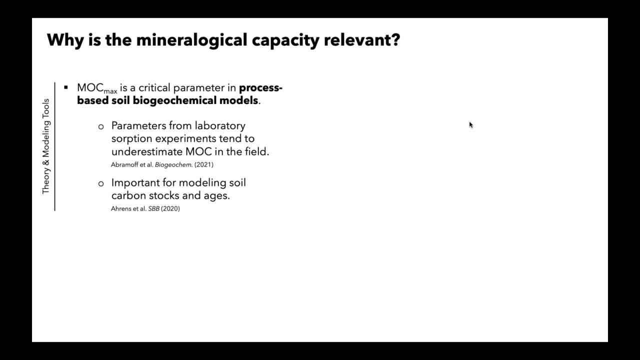 even by order, an order of magnitude, and so getting this parameter right is important for modeling soil carbon stocks and ages. So this is an example of this, But from a practical perspective, it can also inform the potential carbon sequestration efficiency as a function of percent saturation, where you can imagine a soil far from saturation. 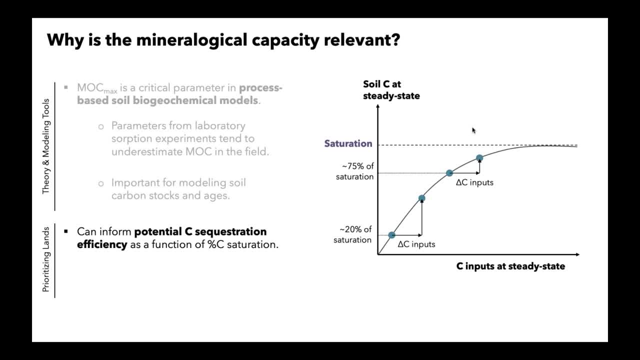 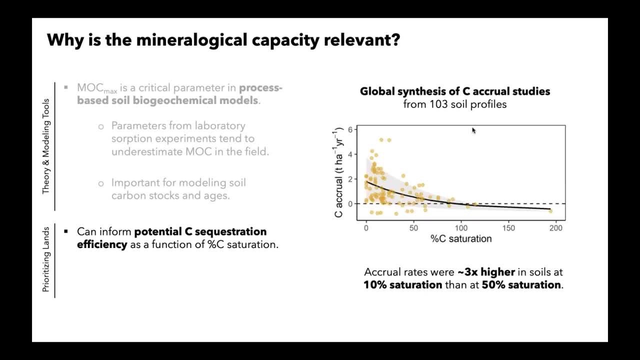 may accrue more carbon for the same change in carbon inputs than a soil closer to saturation. And indeed we see just that. in this global synthesis of carbon accrual studies led by Olga Vendushkova across 103 soil per year, We found that carbon accrual rates were, on average, about three times higher in soils at 10%. 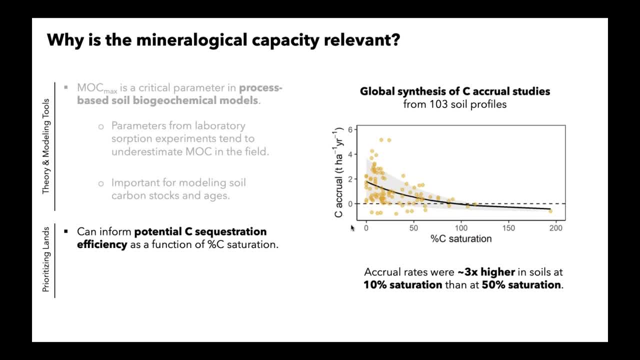 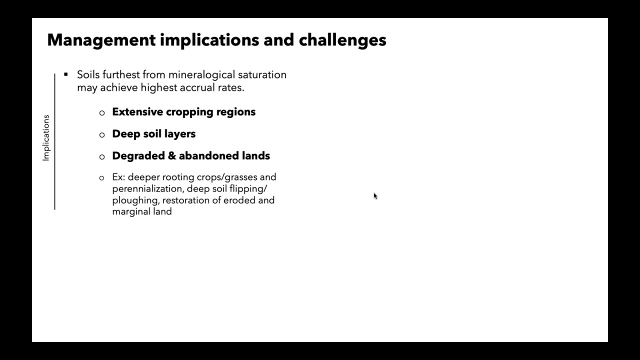 saturation than soils at 50 percent saturation, And so this suggests that this percent saturation can serve as an additional consideration when evaluating and prioritizing lands. So we've shown here that soils furthest from saturation are historically less likely to have. soils furthest from mineralogical saturation may achieve the highest carbon accrual rates. 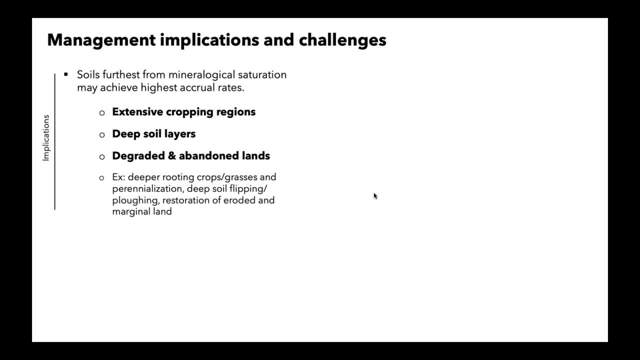 And also our analysis suggests sequestration hotspots, including extensive cropping regions in the Midwestern US, Europe and India that could be targeted for carbon accrual, as well as deep soil layers and degraded and abandoned lands, And there are a number of practices that could be used to do this with a couple of field. 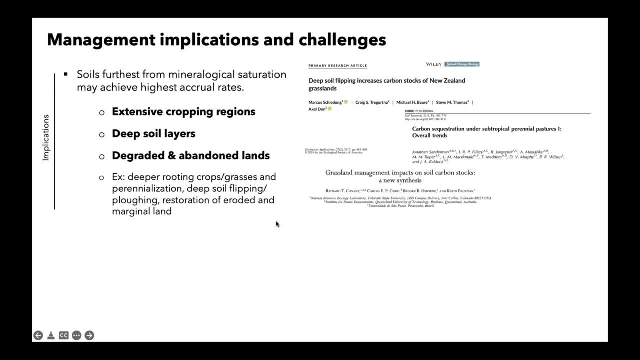 limitations highlighted here, including deep-rooting crops and perennialization, deep soil flipping and plowing at a more extreme potentially, and restoration of eroded and marginal lands. Of course, there are important economical and environmental limitations to consider, with a couple of examples from the literature shown here. 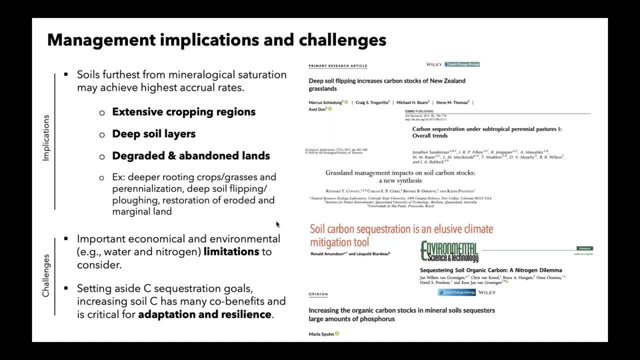 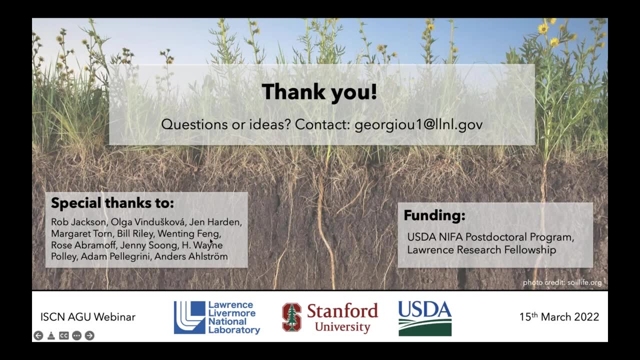 But setting aside these carbon sequestration goals, increasing soil carbon has, of course, many co-benefits and it's critical for adaptation and resilience. So with that, I'm happy to take any questions. A special thanks to my collaborators and to my funding sources. 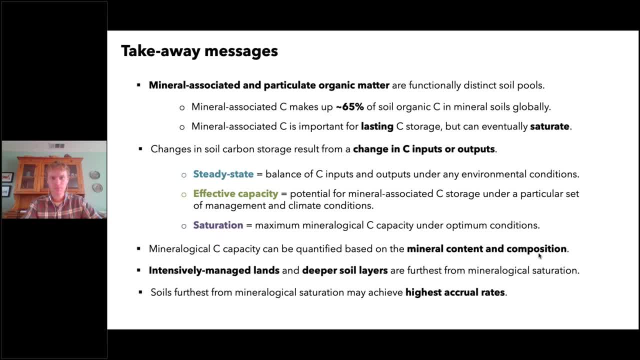 And I can leave this sort of takeaway messages up and take any questions. Wonderful, Thank you, Kat. Right on time, Excellent, Okay, Well, we got some great questions live via the chat function and also some from registration. So let's see how far we get with the time we've got. 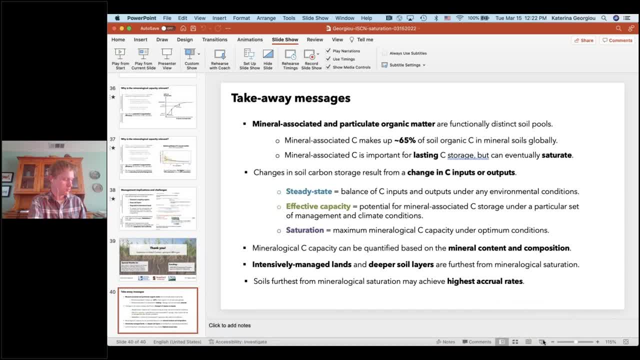 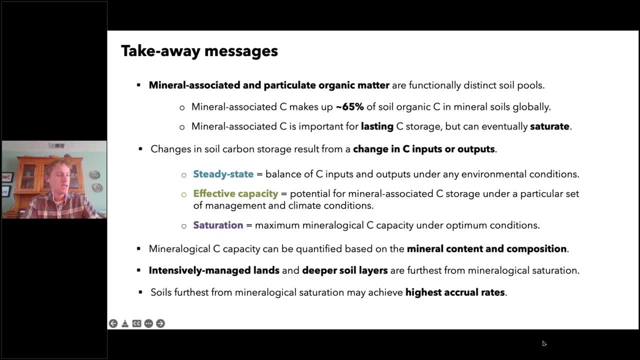 First up, this is a clarification question, but it might be good to address initially. You may have mentioned this in your talk, but perhaps you can touch on it again And it's a good question, Thank you. Thank you, And in your synthesis, how did you define mineral-associated organic matter? 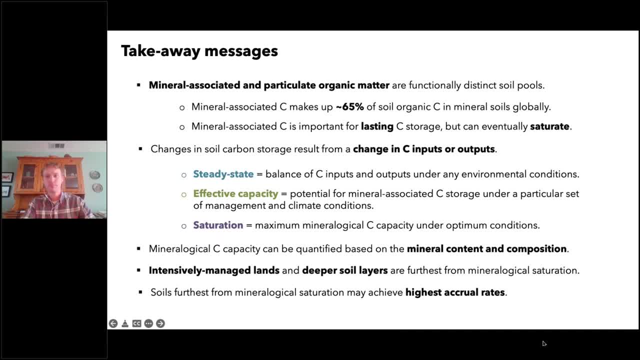 What were the boundaries on that category? Right, That's a really good point. Yeah, For lack of time I didn't go into fractionation in greater detail, But for the synthesis, we did synthesize both density and size fractionation. 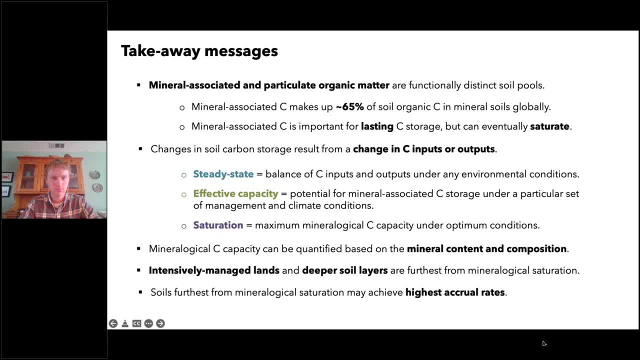 We didn't see any difference. for the purposes of our study between these two, We just took the two methods. But yes, the…so yeah, both fine-size fractions and dense fractions. All right, thanks. So another question that popped up in the chat here has to do with gaps in the data. 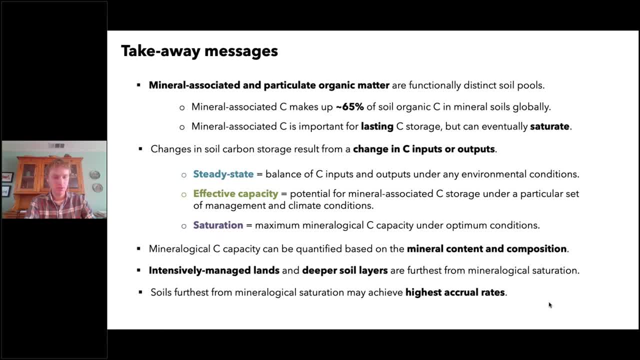 So were there particular soil types or mineralogical contacts that were underrepresented? In particular, this questioner was wondering about low activity clays and how there seemed to be much less data from that category. So does this tell us something about where we ought to focus our efforts? 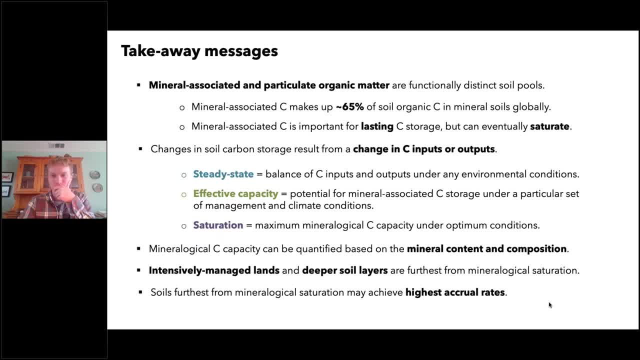 Right, Yes, that's a great question, So it is true. So first, about the low activity clays, it is true that there were fewer points from those regions, also because they represent less global surface area And, of course, we know that the tropics can be data poor. 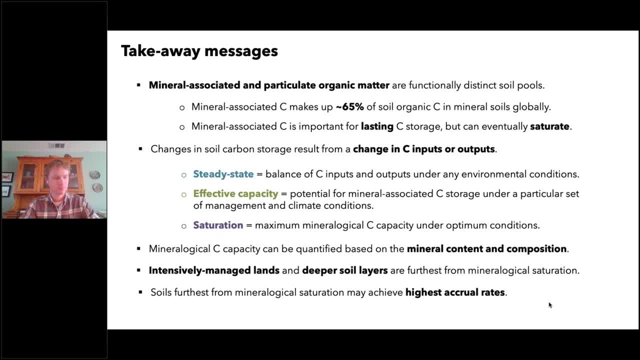 And so, of course, focusing on more sampling, there would be great to further confirm these mineralogical limits or see if we haven't captured the full variability. Also, we played around with additional mineral categories, including non-crystalline minerals, and treating andesols as a separate category. 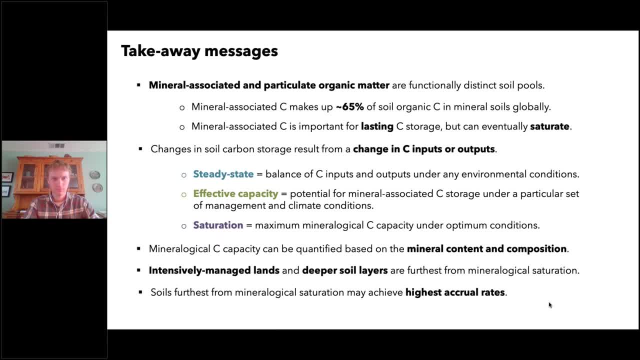 They actually fell within the high activity minerals in our study, But further sampling in these soils would also be great to focus efforts on. Of course, their andesols are about 1% of the global soil surface area, But they do have a large potential for mineral-associated carbon. 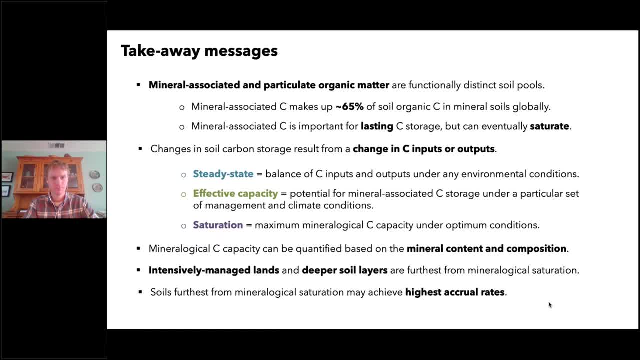 And so, yeah, further sampling in these soils as well would be great. So here's a somewhat related question about how the organization of minerals in space might matter. So this is from Catherine Roche. Okay, So this is a question from Catherine Roche. 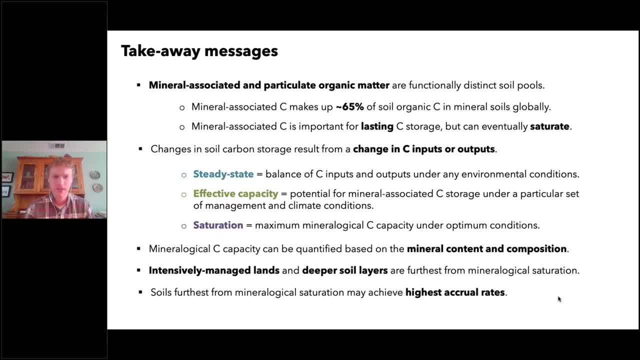 Catherine Roche asks: where do aggregates fit in with carbon saturation? How do you think about this? Right, That's a good question, And so to some degree. so the micro aggregates- well, silt-sized micro aggregates- can also be incorporated in this mineral-associated fraction that we've been looking at. 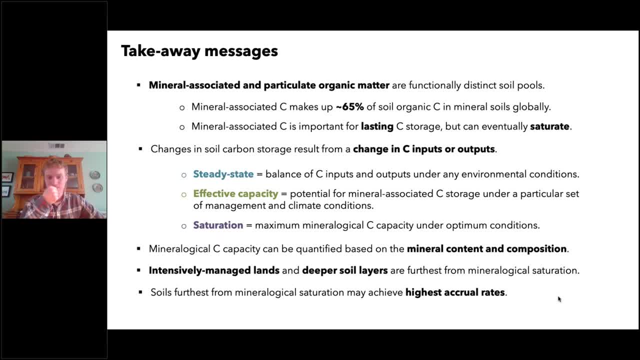 But of course aggregation is not always the answer, And so we're not sure what the answer is. I think aggregation could potentially stabilize even more carbon that we haven't really focused here from this mineralogical lens. So, yeah, I think I mean, yeah, aggregation is very important. 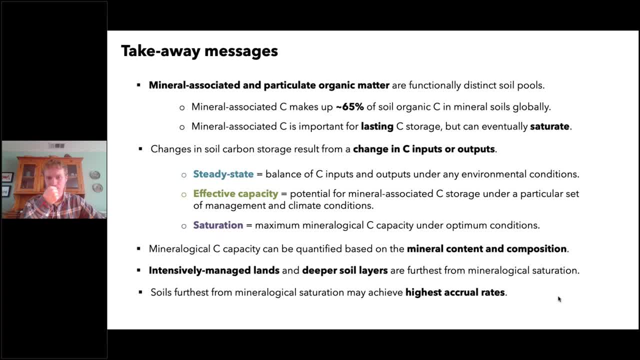 And it potentially could lead to even more carbon storage, But that wasn't a focus of our study from this particular mineralogical lens. Now I wonder: is it? to what extent is it implicit in the synthesis? as you've already done it, 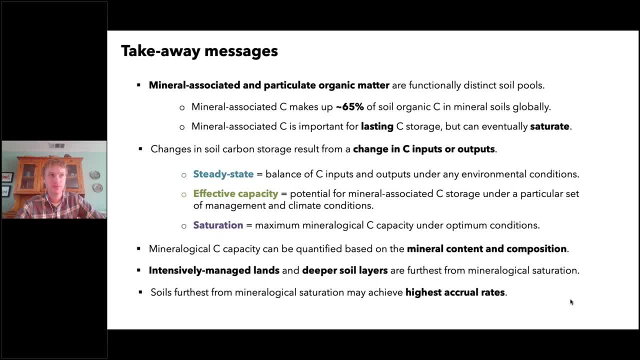 Or would it require considering an aggregate occluded fraction separately? Yeah, I guess it would. it could be interesting to look at an aggregate occluded fraction separately as well. In the synthesis as we have it and have used it, the sort of silt-sized micro aggregates. 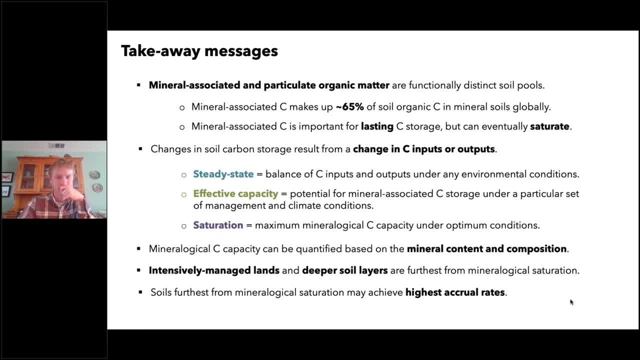 would also are also included in driving these limits. But yeah, I think it could be worth looking at the sort of aggregate occluded fraction separately as well And there have been studies that have sort of done this. but that would be interesting sort of at this global scale as well. 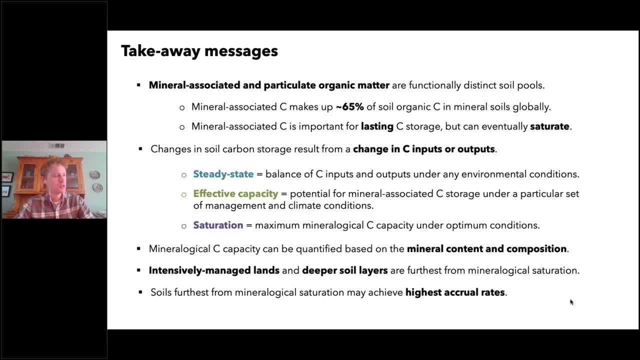 Cool. Here's one question that was actually submitted during registration, but it seems like an especially important one, so I'll pose it now. How do you think climate change could affect the patterns that you were just discussing? Is this something we need to consider? 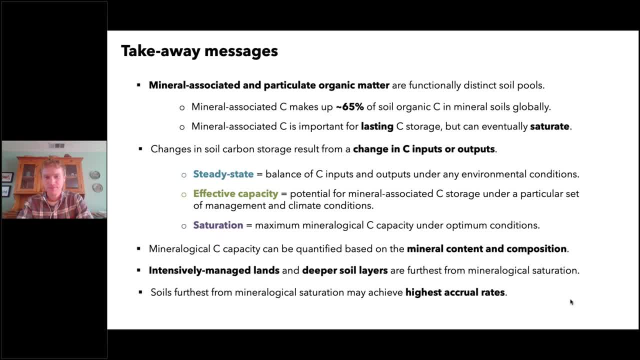 Yeah. So, as I showed briefly with regards to climate, we do find that we do predict that increasing temperature will could lead to losses in mineral associated carbon as well, So it certainly could cause a departure from saturation or make it even more difficult. 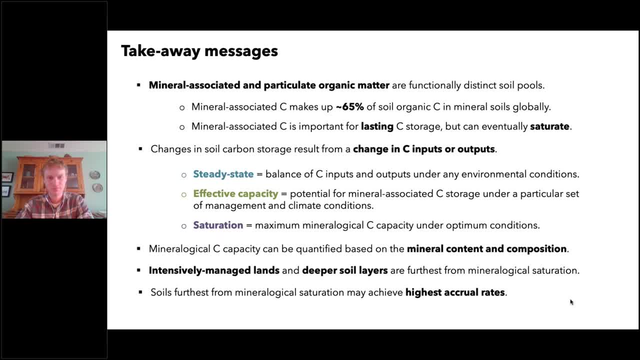 to approach. So, yeah, it can certainly play an important role in achievable limits. Yeah, But also, as we saw this, we found that the soils closest to saturation were also- at least using this statistical model- were also potentially more resilient to losses. 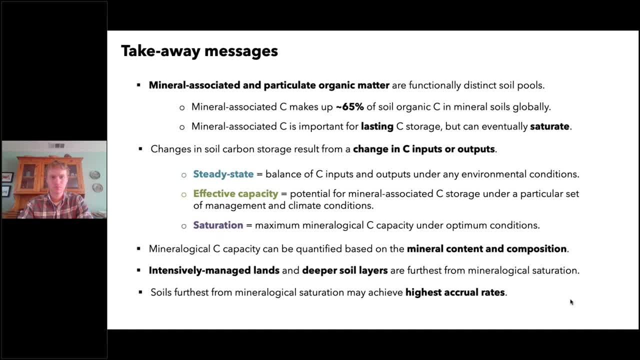 And so Yeah. So yeah, there could be trade-offs there where where sort of building soil carbon could lead to more resilience and fewer losses with climate change. All right, Well, we've got time for maybe another one or two questions. 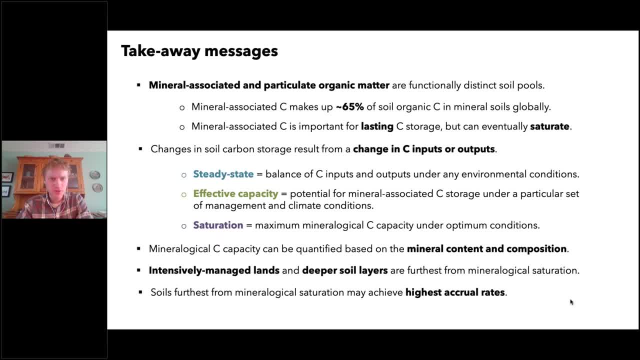 So there are some interesting ones about microbes in here, So let me see if I can find this one again. If I can paraphrase here: So can we really compare shallow and deep soil, given the different microbial community and input rates in those two environments? 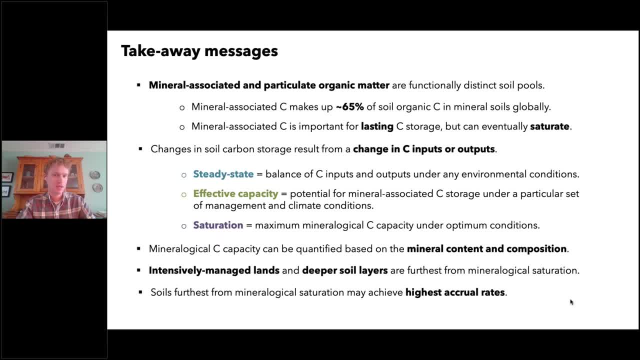 So what? how does, how does the biological factor come into play here? I'm, yeah, I mean, I guess it depends comparing them in. in in what respect? So I guess I mean comparing them in terms of their mineralogical saturation, it's, it's. 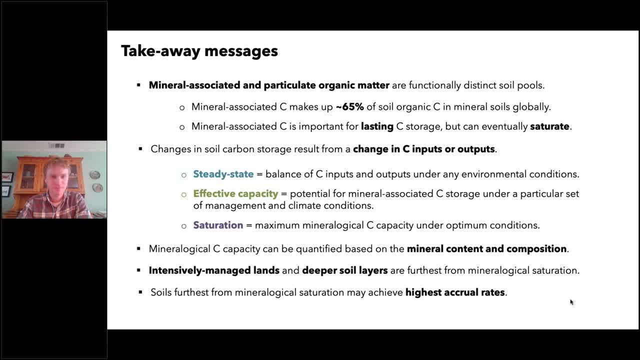 certainly true that deeper soils are very far from it and and likely quite difficult to to reach, though it's still relevant, as nicely demonstrated from a modeling perspective by the paper that was cited in a previous slide in 2020.. So I guess- yeah, I mean certainly we, we should, we can. I guess what I'm, what I'm trying. 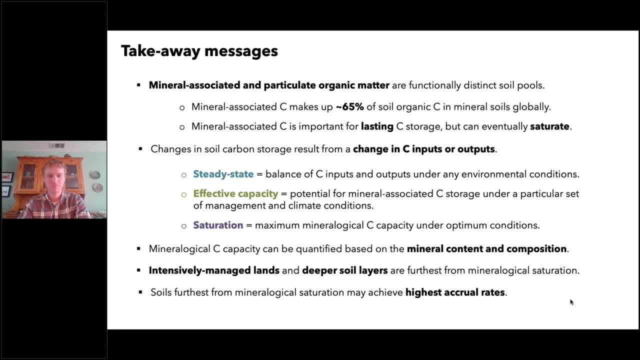 to say is that, from a mineralogical limit, I think it's still relevant to both soils. It might be very difficult to to reach in deeper soils, but it still can be relevant for prioritizing one deep soil versus another or, in the case of modeling, it can be very 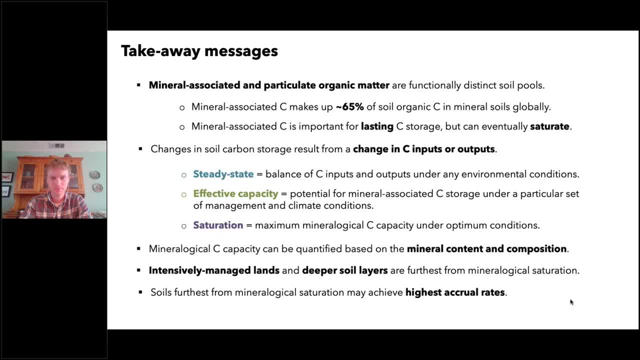 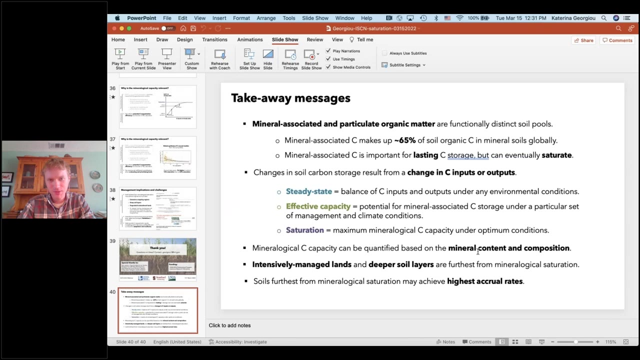 important, But certainly there are differences, and it's it can be difficult to reach saturation in deeper soils. All right, Well, let's see we should probably move on to our next speaker now, although there are many tempting questions in here, but perhaps they can come up at the end. 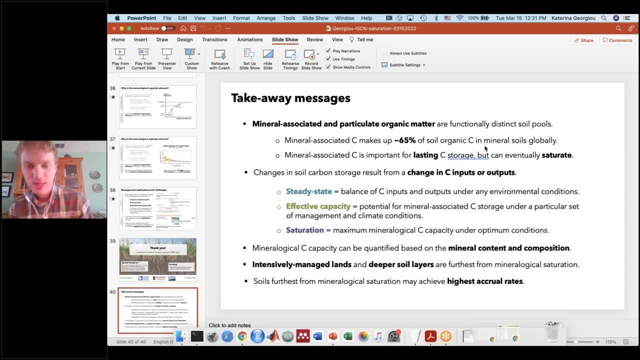 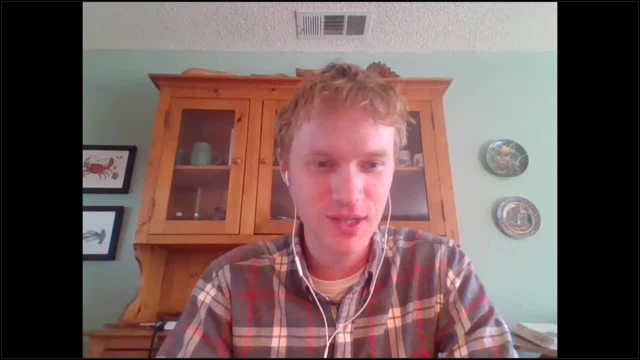 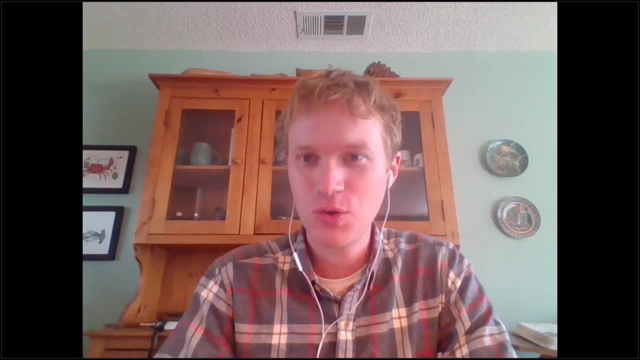 Thank you very much, Kat. That was a that was a wonderful primer on this topic And and that that research you've presented is. it's exciting every time I hear about it. So many thanks, Thanks so much. We're going to shift to our second speaker now. 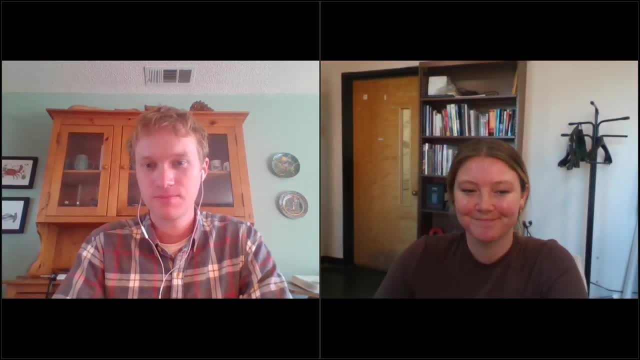 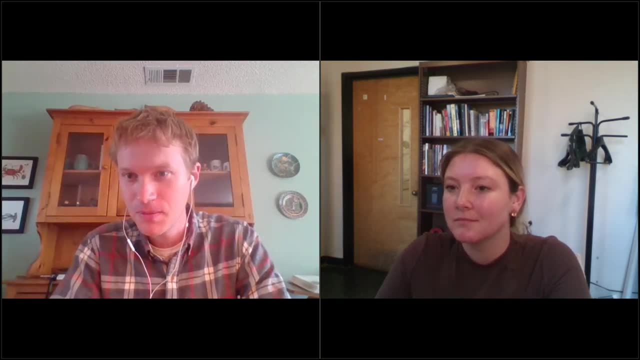 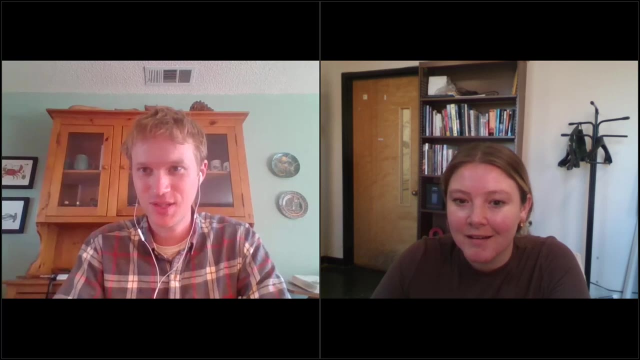 This is Maura Slocum from University of Pennsylvania, And let's see, do I need to do something here? I probably do Make presenter Excellent. Thank you, Excellent, Yeah, Great, All right, Just a second here while we boot up. 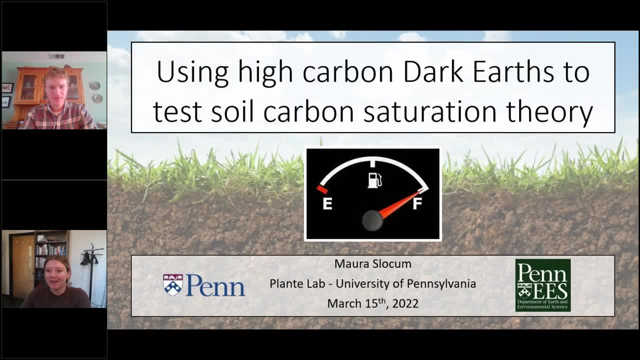 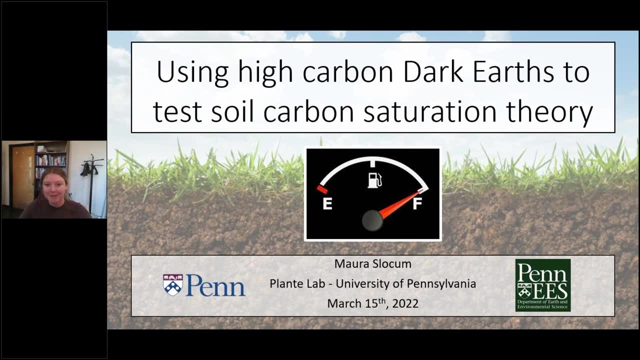 How are we looking? Can you see that, Eric? Yeah, it looks, looks great. Okay, All right, Maura, take it away. Awesome, Thank you. Thank you to both Kat and Eric. I'm very excited to continue the conversation today about soil carbon saturation. 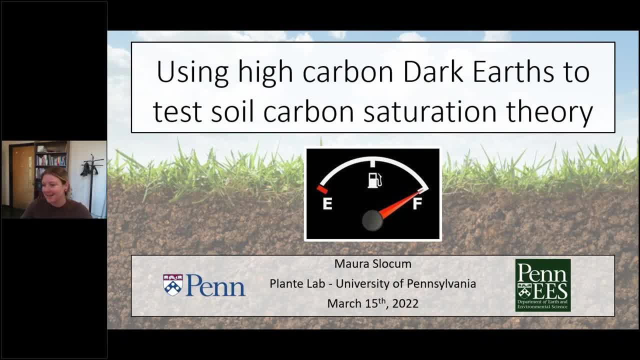 So, yes, my name is Maura. I'm a PhD candidate at UPenn in the FONT lab, And in this part of the session I will be exploring carbon saturation theories using high carbon soils called anthropogenic darkers, And I appreciate that we are coming together from different backgrounds and that soil carbon 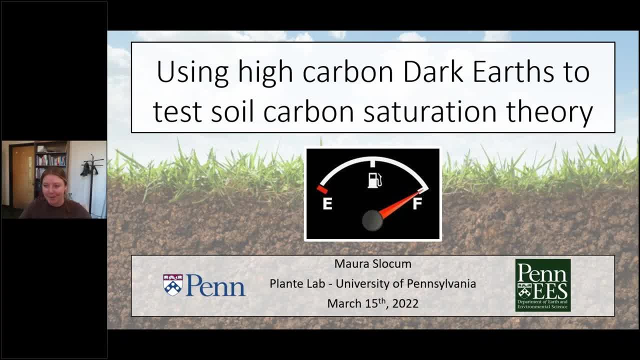 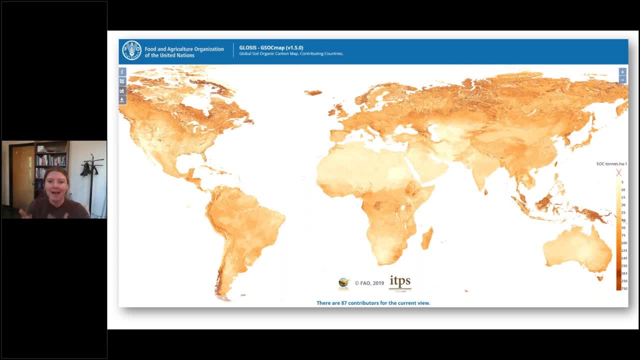 sequestration is very much a relatively hot topic right now. So I want There Is a very heavy burden being put on soils when we think about soil carbon sequestration, And here I have a map from the Food and Agriculture Organization of the UN. 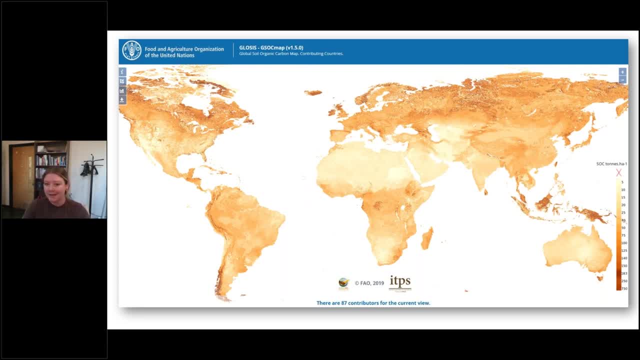 They put together this global soil organic carbon sequester sequestration potential map, which is a mouthful but has the more easily accessible name: GSOC SEC V 1.00.. But anyways, this map seen here shows estimations of soil organic carbon sequestration potential. 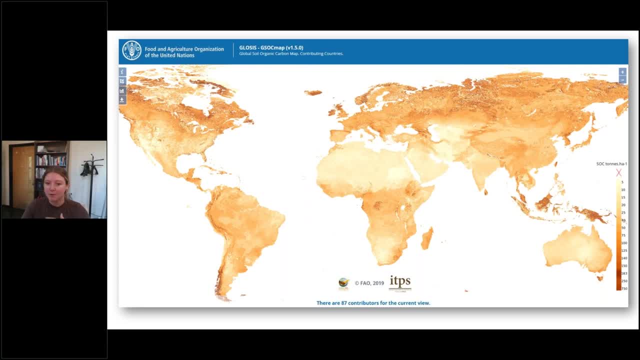 for topsoil under different managed soil management scenarios, And these scenarios include five to 20% increases in carbon inputs to the topsoil And, as Kat showed us, increasing inputs might lead to soil carbon saturation. So to better understand. So better understanding of soil carbon saturation and the theory behind it will help us estimate. 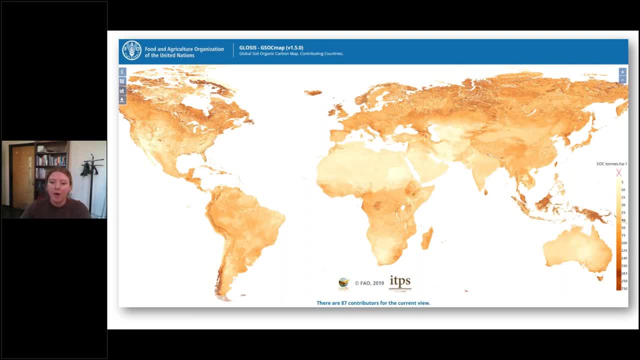 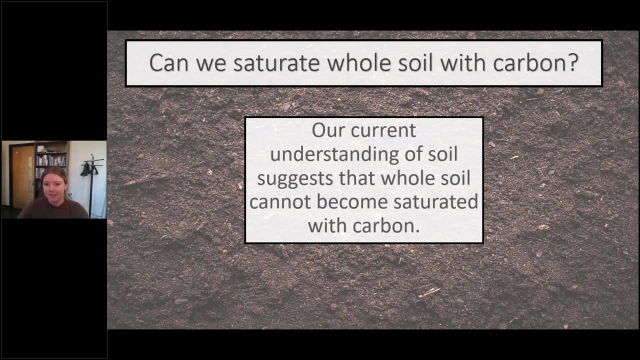 the use of soil as a method of carbon sequestration. So soil is a complex system, So we should be sure to orient ourselves appropriately when discussing soil carbon saturation. When we're out in the field, we Often can see soil as a whole entity and it's natural to wonder whether that, whether 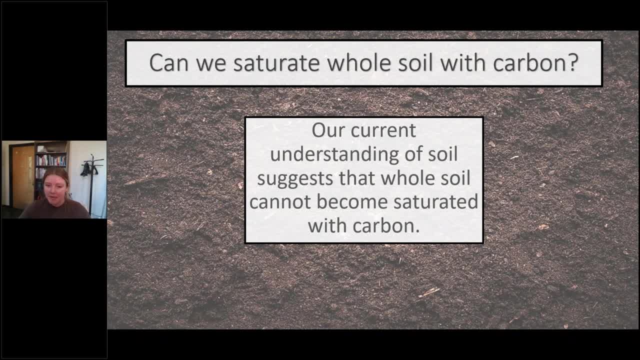 whole soil can be saturated with carbon, But based on our current understanding of soil carbon dynamics, it does not seem that whole soil can become carbon saturated. So I wanted to break down what that means and what we are looking at when we're considering this question. 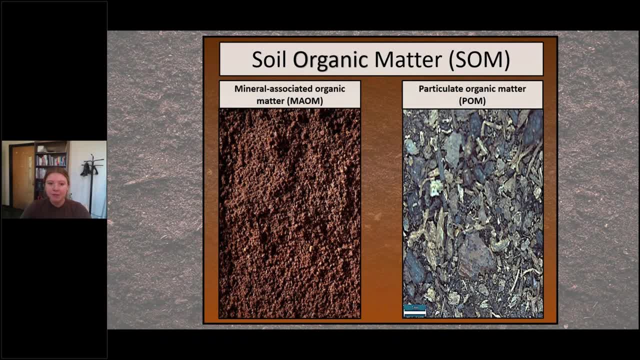 So, although soil organic matter Only makes up between two to 10% of the soil's mass, we know soil organic matter holds a large, large portion of Earth's carbon And, as Kat mentioned as well, soil scientists have categorized soil organic matter into: 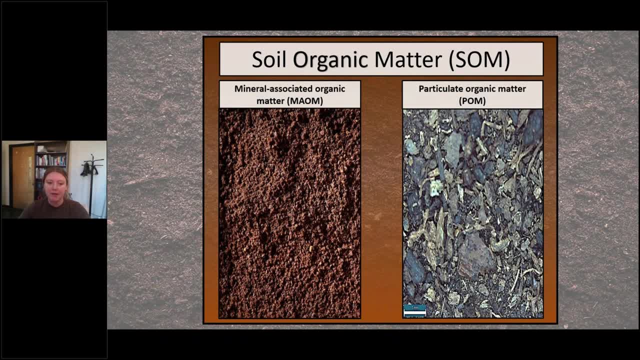 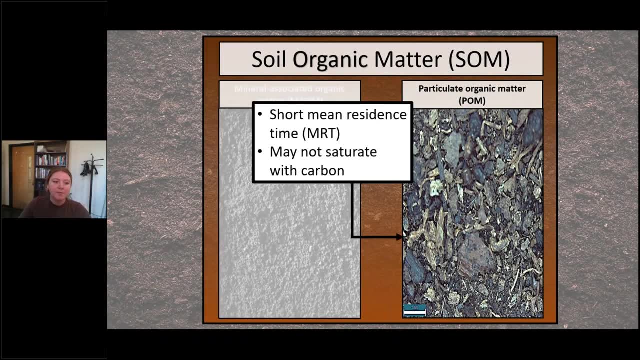 different pools, including the mineral associated organic matter and particulate organic matter. And particulate organic matter typically consists of Decomposed detritus and plant material and is often considered readily decomposable and therefore soil organic matter is assumed to have a shorter mean residence time in this. 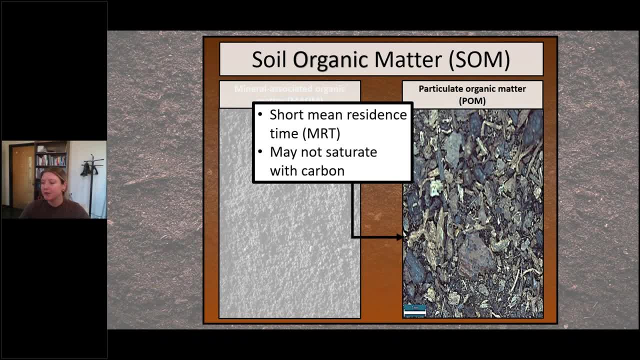 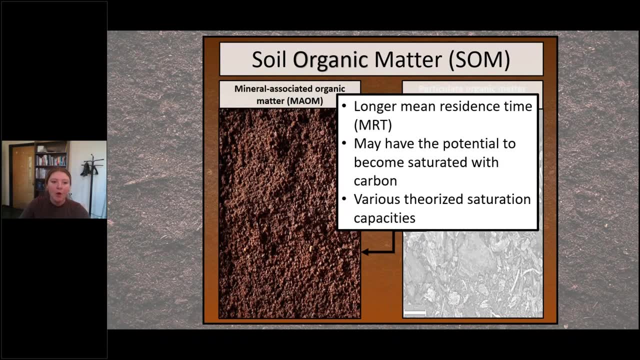 pool And particulate organic matter is considered a very dynamic pool and may not have the capacity to become carbon saturated, While mineral associated organic matter is considered more persistent and has that longer mean residence time. Organic matter that is mineral associated typically consists of more organic material. 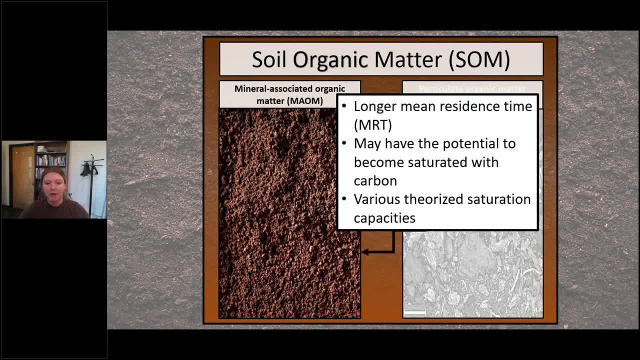 that has been chemically transformed by soil biota And, due to the adsorptive relationship between soil organic matter and a soil mineral mineral, associated organic matter is less accessible to decomposers And, as Kat mentioned, soil carbon saturation may be achieved. 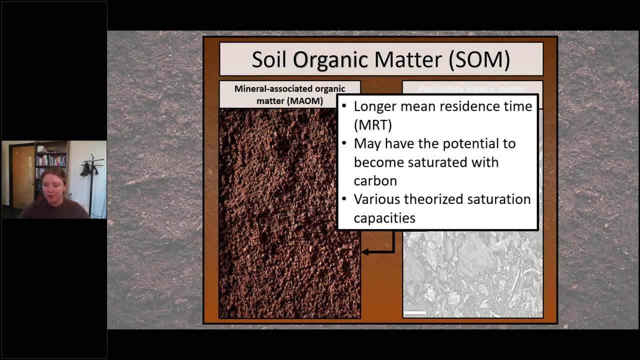 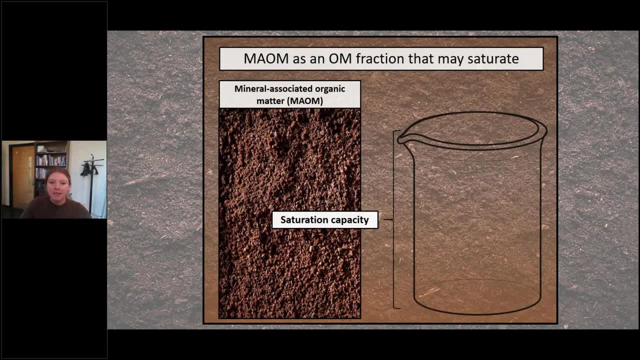 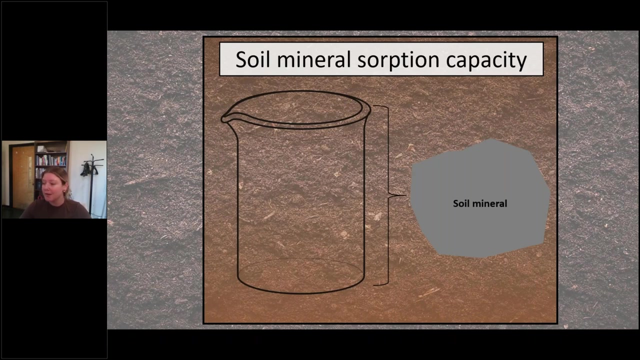 When any additional input of carbon into soil results in no increase in mineral associated organic carbon. This limit has been explored by soil carbon researchers and the upper limit of mineral associated organic matter may be considered as the theoretical capacity for soil carbon saturation If we imagine all the soil mineral surfaces available for organic matter adsorption within. 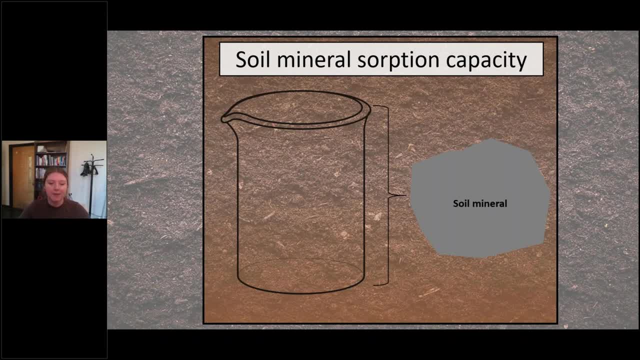 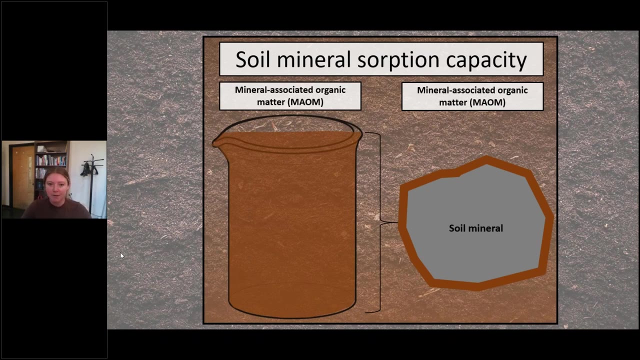 a soil, we can theoretically quantify the capacity of that soil to become carbon saturated, And I've represented this capacity here by a beaker. If every available soil mineral surface is covered by adsorbed organic matter, then we may consider the mineral associated organic matter pool. 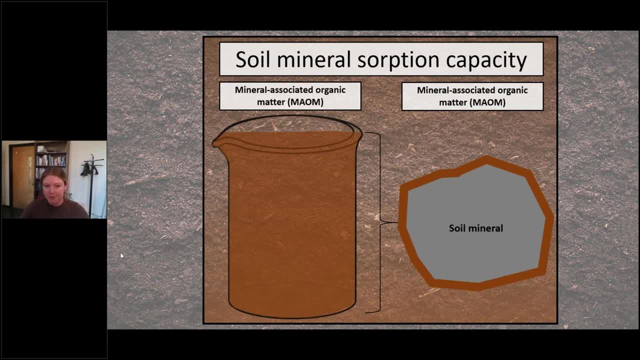 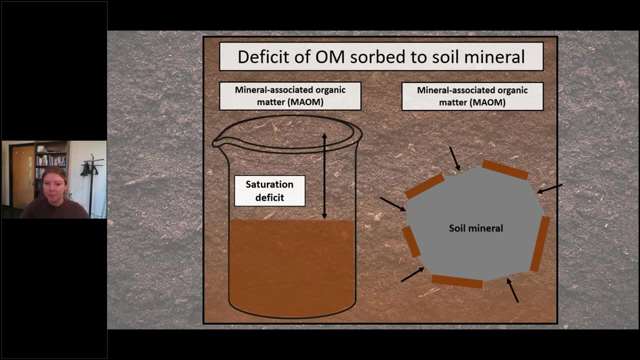 And we can also consider the mineral associated organic matter pool as fully saturated with soil carbon. But if only some of the soil mineral surfaces are covered with adsorbed organic matter, then we might say that there is a saturation deficit. Any additional input of organic carbon could find its way to those open spaces and reactive 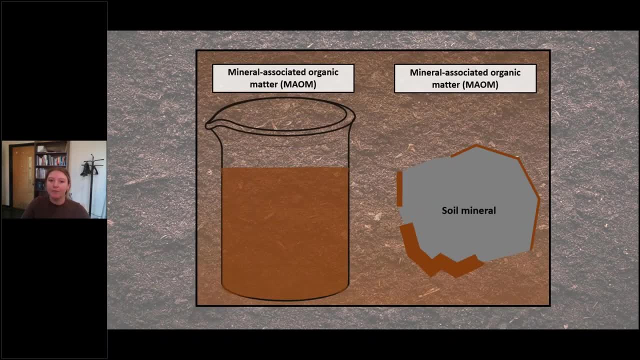 soil mineral surfaces. We believe, however, that organic matter does not absorb to the soil mineral surface uniformly. Mineral associated organic matter can be patchy or appear as clumps on the soil mineral surface And this can make it difficult to theoretically quantify soil carbon saturation in the mineral. 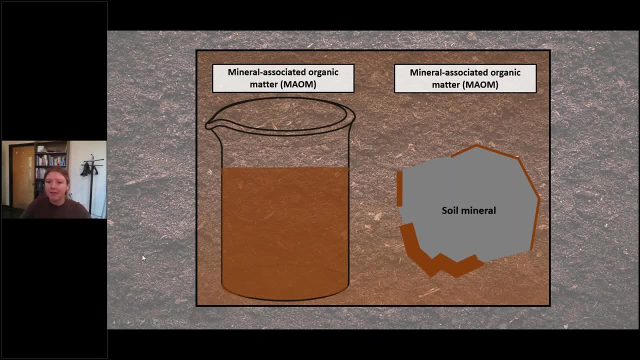 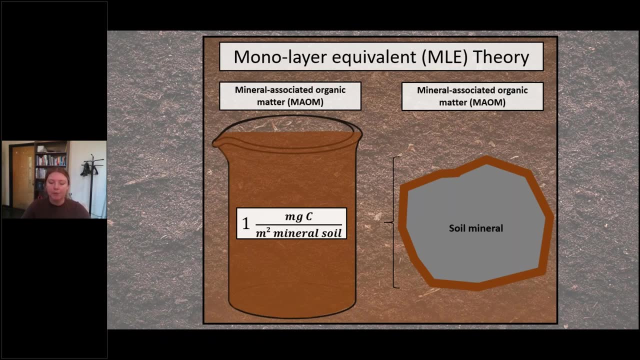 associated organic matter pool. So, based on the former conceptualization of mineral associated organic matter, Lawrence proposed a limit for mineral associated organic matter based on studies done on the relationship between the surface area of marine sediments in a continental shelf and the associated organic carbon. 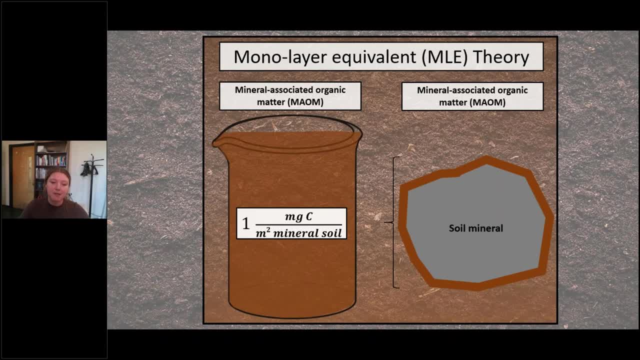 The relationship between soil carbon and soil mineral surfaces was conceptualized as this monolayer equivalent. This allowed us to produce a quotient that relates the concentration of carbon to the surface area of soil minerals, And the limit proposed by Mayer using this quotient is one. 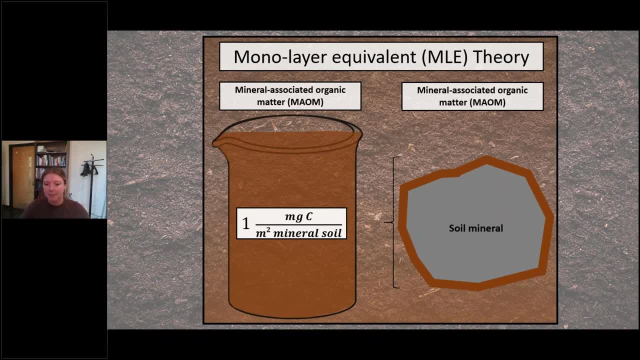 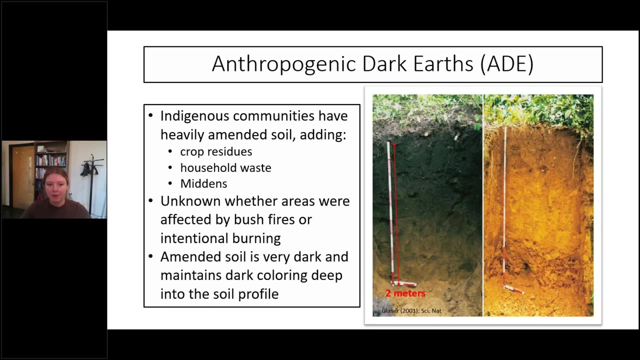 However, there is limited research on how this theorized limit holds up when put to the test in soils. So that's what I've been doing in the Plant Lab, So I've been working with soils that may be saturated with carbon, anthropogenic darkers. 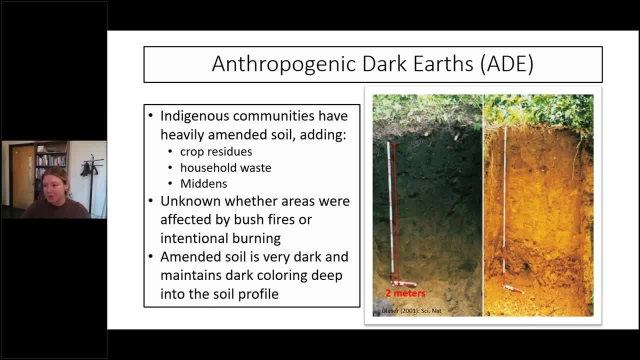 And these are soils that have been amended by indigenous communities and regional populations all over the world, including the Amazon, New Zealand and West Africa, And studies on Amazonian darkers have shown that the soil remains dark, with high carbon concentrations deep into the soil profile. 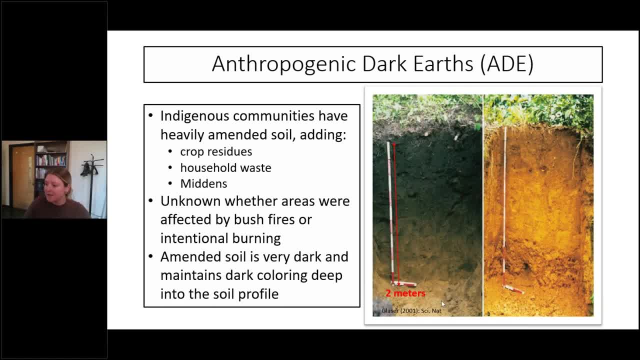 Here you can see the color contrast between the Amazonian darkers, more commonly known as terra preta, and the adjacent unamended tropical soil. And Amazonian darkers, the terra preta, have been studied extensively, But the communities actually that live near these dark earth locations are not actively 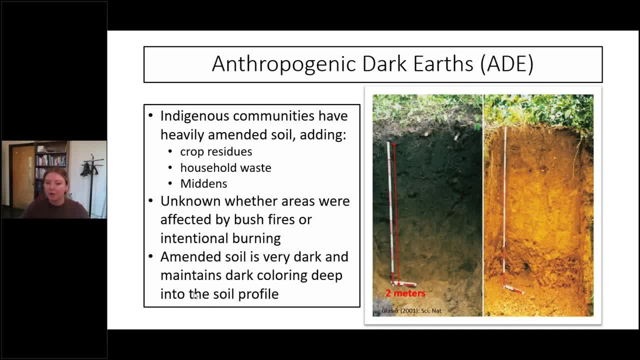 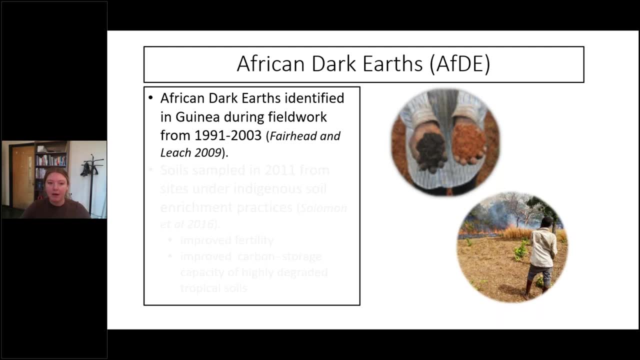 managing the soil. So there are still questions about terra preta's creation, And it is not clear how long ago the soil management that created these dark earths ceased. However, studies have shown that dark earths found in West Africa may be actively managed. 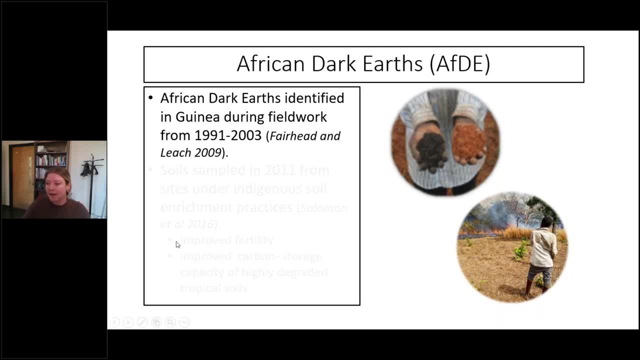 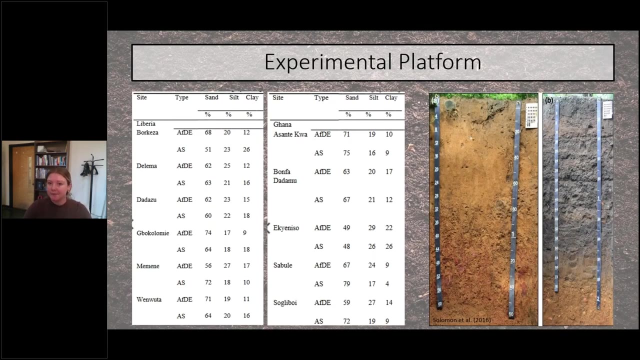 by the communities that live near the dark earth sites, And analysis of dark earth samples show that these soils exhibit increased fertility and may improve carbon storage capacity for these tropical soils, And so I have a case here of soils that have been managed in a way that may be maximizing 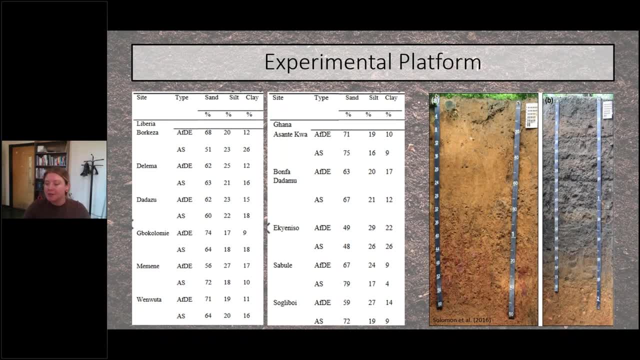 their carbon storage capacity, potentially reaching carbon saturation, And so, using dark earth samples that were collected in 2011 from six sites in Liberia and five sites in Ghana, I isolated a subset consisting of four depth profile pairs. Each pair is an experimental platform that allows for a comparison along the soil profile. 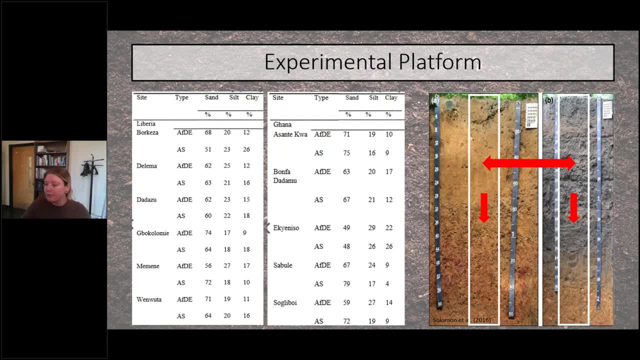 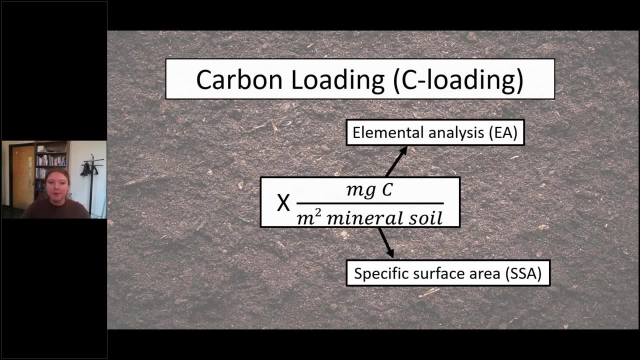 and between a dark earth profile and an adjacent profile of the unamended soil. So, using this platform, we can use samples that were collected from 15 centimeter increments along each soil profile to measure and calculate the carbon loading value that Kat mentioned. 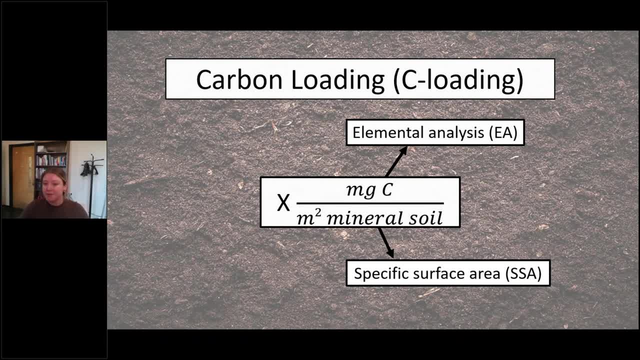 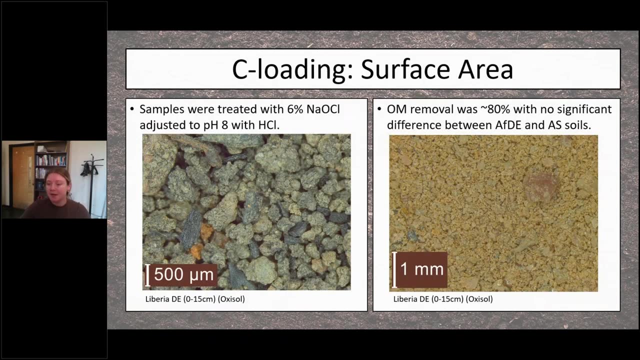 otherwise known as the quotient relating carbon concentration to soil. mineral surface area, And carbon concentrations were measured here at Penn using elemental analysis and gas chromatography. Soil mineral surface area was measured after samples were treated with a sodium hypochlorite solution, which removed about 80 percent of organic matter from both the dark earth and 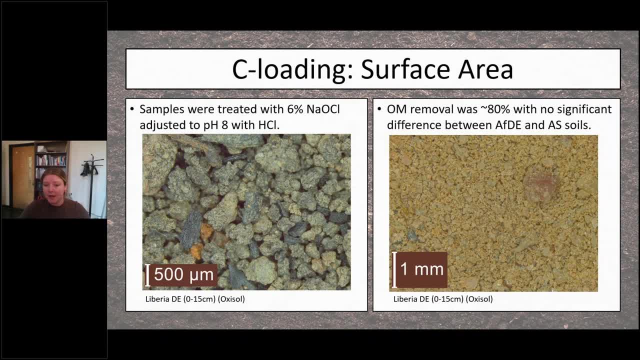 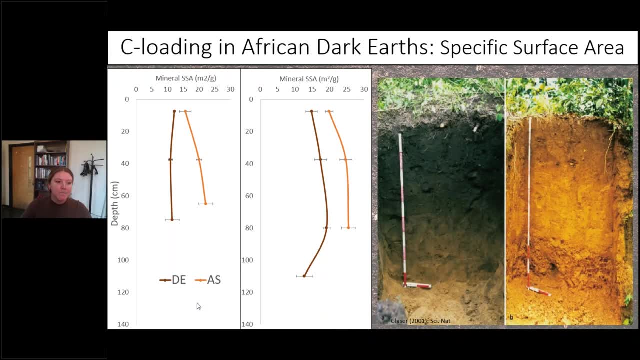 adjacent soils, And this organic matter removal process allowed us to measure the soil mineral surface area. So here we have the results of that surface area analysis and these are two representative profile pairs. The dark earth profile is in dark brown, while the unamended adjacent soil is represented. 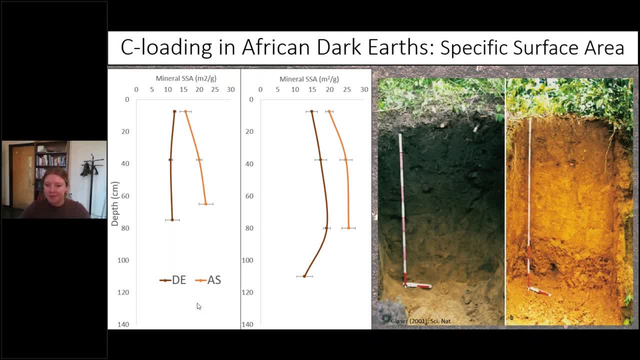 by the brighter orange color, And both of these soils have relatively low mineral surface area and the differences between the soils may be due to the incomplete removal of organic matter. So after getting these surface area values, we considered looking at just the clay mineral. 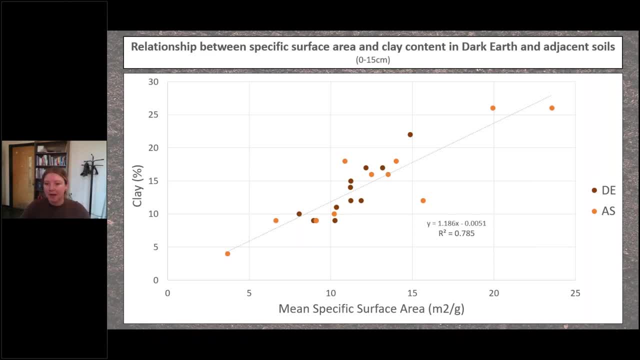 samples And we found that the clay minerals are the most reactive soil minerals, because it's important to remember that typically the most reactive soil minerals are the clays And what we see here from a comparison of surface soil from all 11 sampling locations. 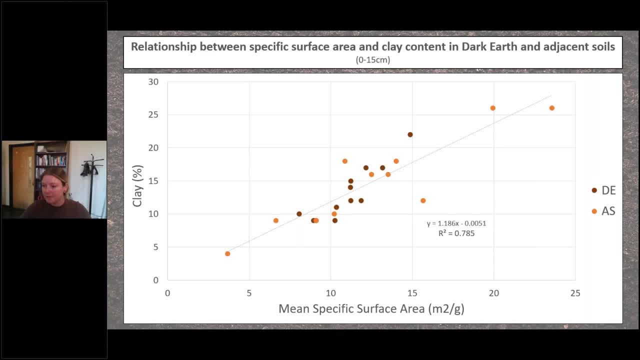 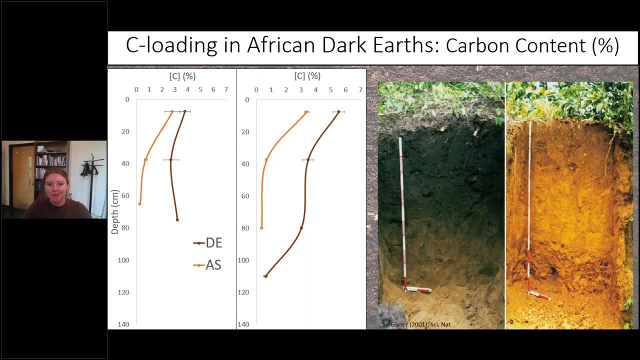 we see that clays are driving those specific surface area values regardless of soil amendment. So the next step is to look at soil carbon concentrations, And we see here that even at depths greater than half a meter, dark earths contain greater amounts of carbon compared to that unamended adjacent tropical soil. 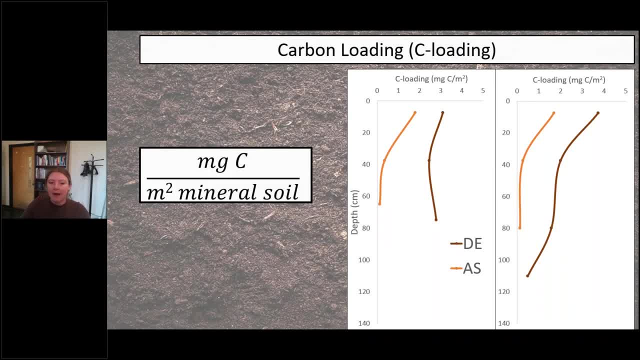 And so, now that we have the surface area measurements and the carbon concentrations, we can use these measurements to calculate carbon loading, And from these calculations we see that dark earths exhibit greater carbon loading and, in other words, have more carbon per square meter of soil mineral surface compared to. 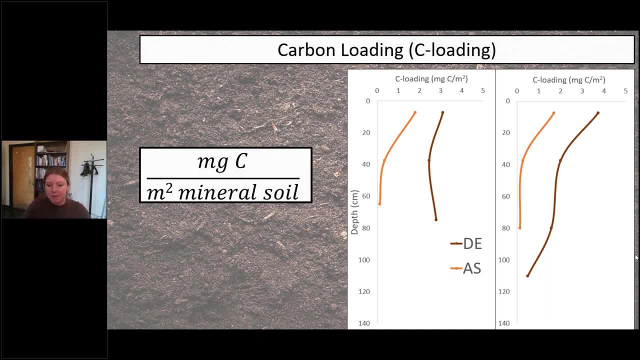 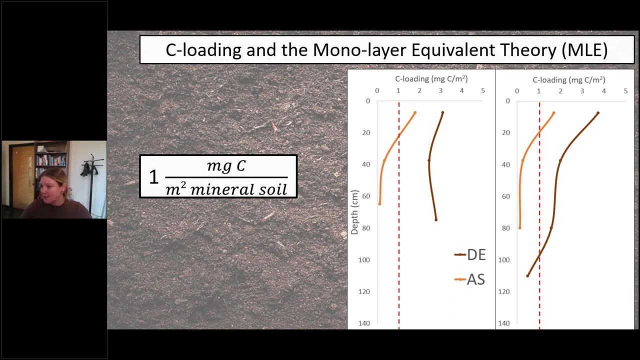 the adjacent unamended soil. But what is most interesting to me about these results is how these values compare to that monolayer equivalent theorized limit that I mentioned before. So remember that theorized limit is one and we see that the dark earths are well above. 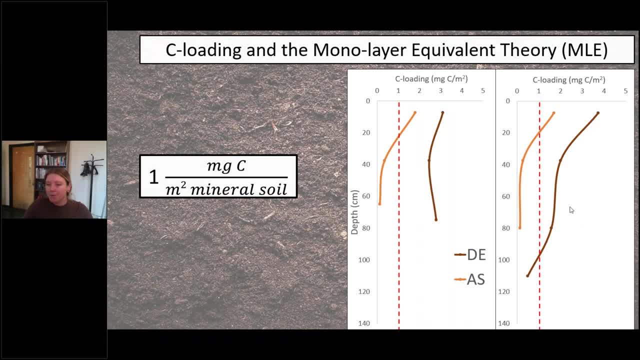 this theorized limit, even as deep as almost a meter. Even at the surface, both the adjacent and unamended soil and the dark earths are above this threshold. Therefore, it could be possible that the limit for this quotient, the limit for mineral-associated 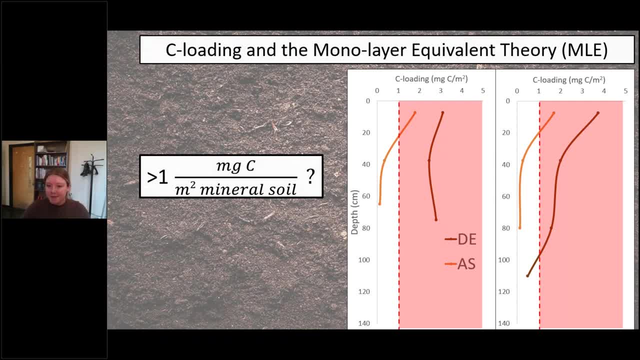 organic matter is above one And if so, what is the limit? And are dark earths at this limit? So if, in other words, the dark earths are above this threshold, then what is the limit? Because if African dark earths are saturated with soil carbon, could they help us understand? 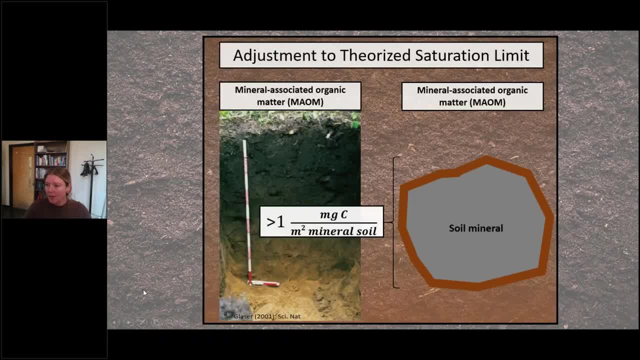 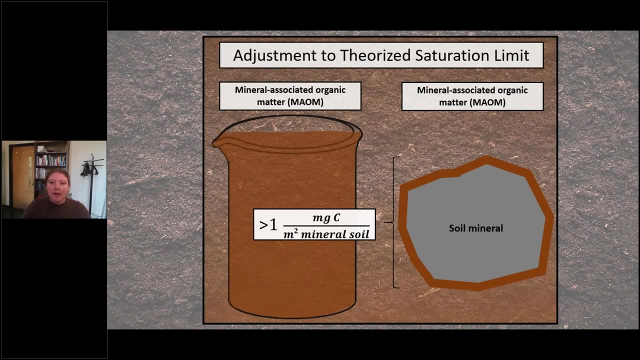 the limit of soil carbon saturation. This isn't to say that the monolayer equivalent concept isn't helpful, but when thinking about that full beaker or the saturation capacity, it may be bigger than we thought And actually the size of the beaker or the saturation capacity may vary. 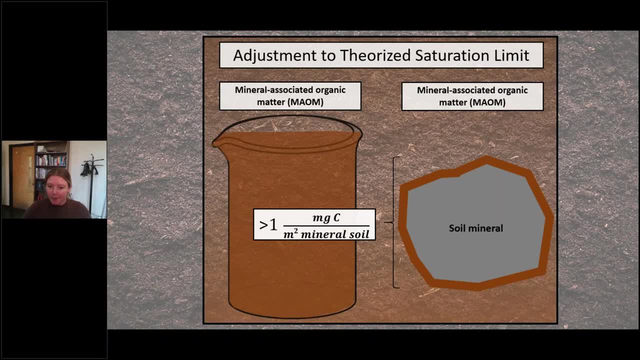 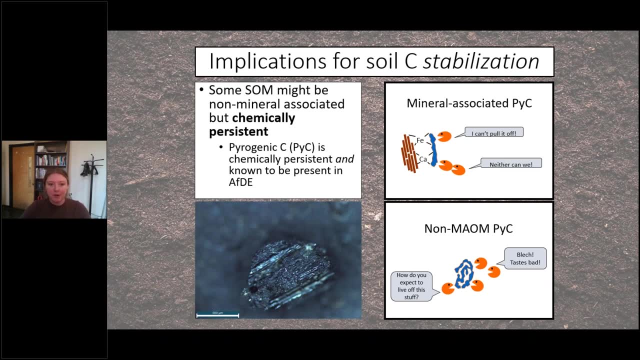 Depending on the soil, as Kat was describing, And but- and there's always a but- I don't want to forget about another exciting characteristic of the dark earths, which is the presence of pyrogenic carbon, And remember that these dark earth locations, they experience some burning, whether intentional, 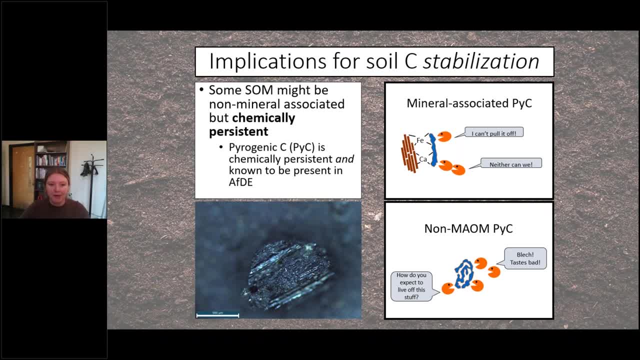 or not that is left behind partially combusted organic matter, otherwise known as char or pyrogenic carbon, And pyrogenic carbon is often found In that particulate fraction. But remember that particulate organic matter typically has a short mean residence time. 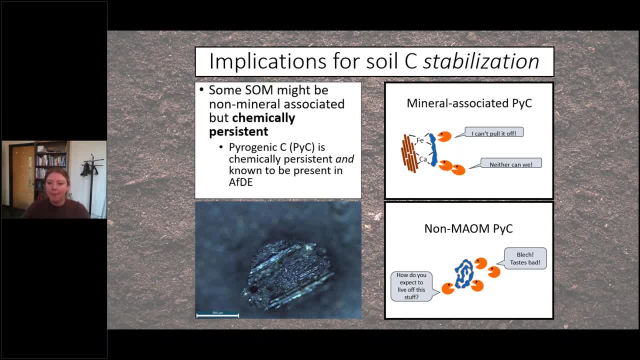 and is considered readily decomposable, While pyrogenic carbon found in the particulate fraction has a longer mean residence time and it's definitely not readily decomposable compared to other particulate organic matter. So pyrogenic carbon, or char, is important in the conversation. 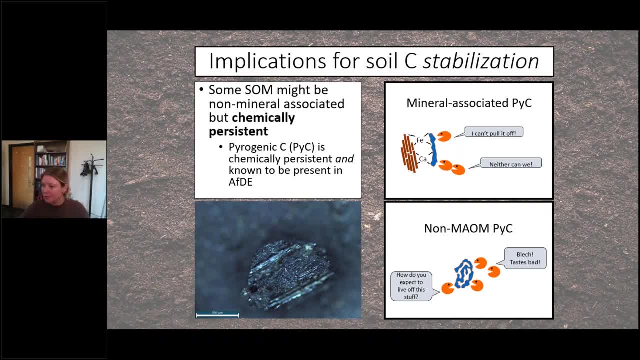 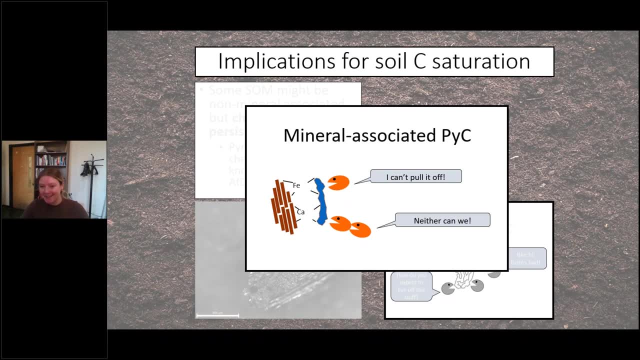 Around: soil carbon stabilization and soil carbon sequestration, And another, but it is particularly interesting to think about pyrogenic carbon, that is, in the mineral associated fraction. So preliminary results from a density fractionation procedure that I performed indicate that there is pyrogenic carbon in the mineral associated fraction, not just in the particulate fraction. 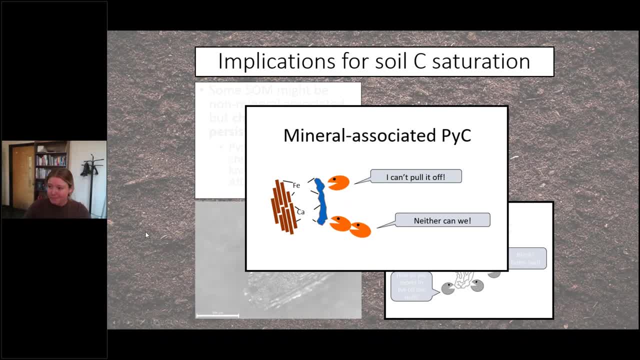 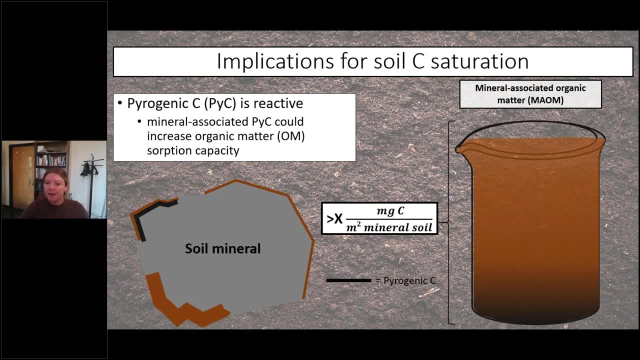 In these African dark earths. So, knowing that pyrogenic carbon is often reactive, if there is mineral associated pyrogenic carbon, this could increase the organic matter absorption capacity of minerals and soil. This increases the size of the beaker or the saturation capacity beyond the surface area. 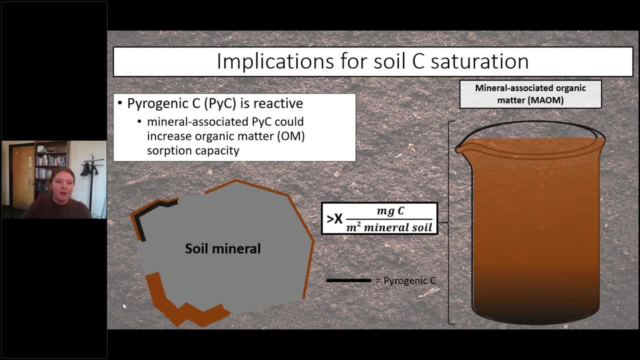 of the soil mineral. So, in summary, do soils have a carbon storage limit? It appears that whole soil cannot be carbon saturated, but carbon storage may be maximized in the mineral associated fraction And it is important to clarify that we can add organic material to soil, increasing inputs. 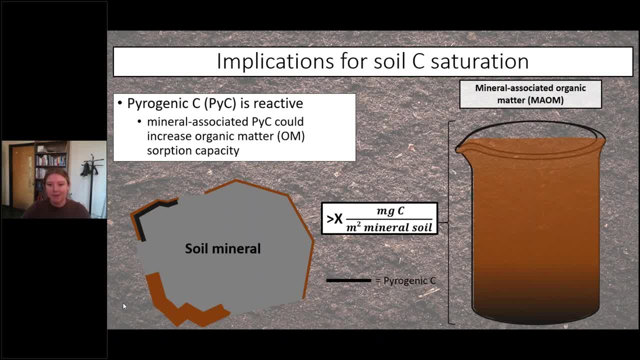 But if a soil is at saturation, those inputs might be shorter lived and not remain in the system for as long as we would like. And what are the parameters that control the mineral association of organic matters? We discussed today how these controls include the sorption capacity of the soil. mineral 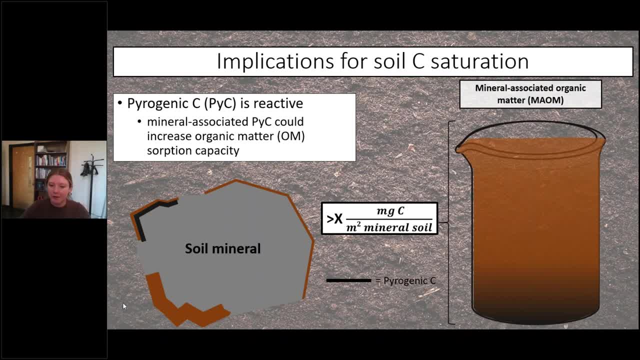 surface, as well as the chemistry of organic matter that sorbs to the mineral surface. So there are still unanswered questions about the saturation capacity of soil and the use of soil and carbon sequestration initiatives, which is why we're here today, And so I look forward to seeing continued feedback. 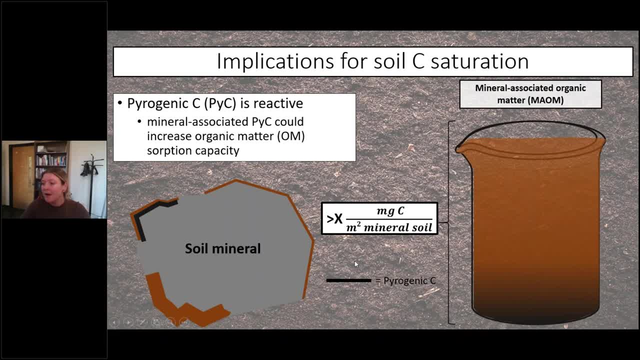 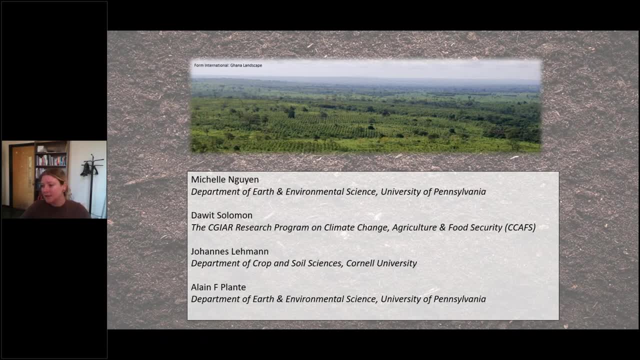 And I look forward to seeing continued research that's done in this field. So that concludes my talk, But I'd like to thank my collaborators, including my lab group members and external mentors, as well as my PI, Dr Alain Plante, who is truly the man behind the curtain. 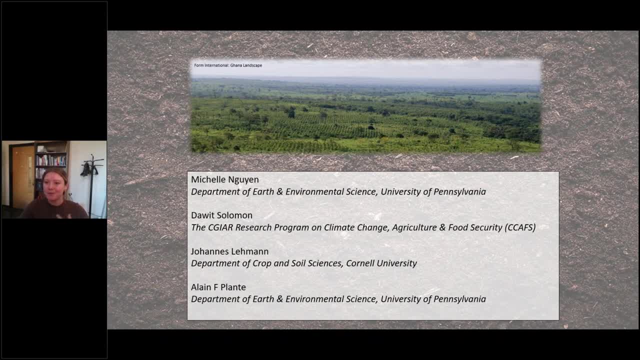 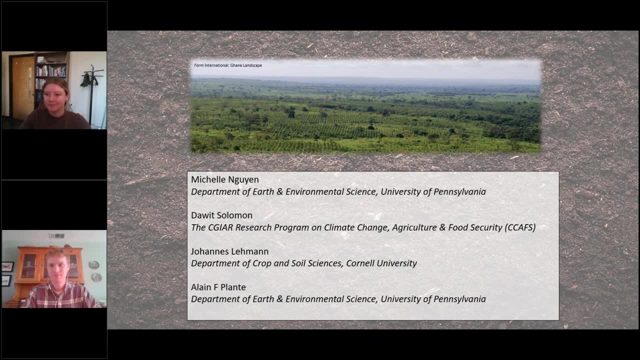 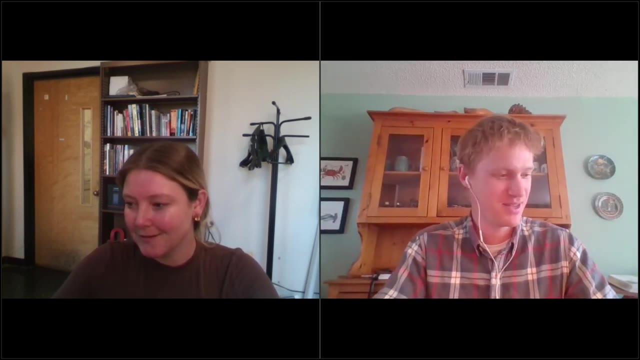 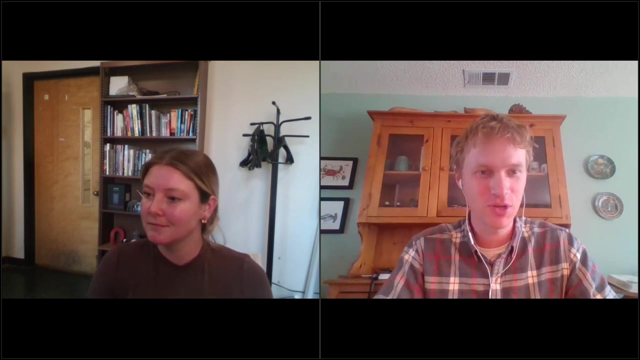 So thank you for coming And I look forward to hearing your questions. All right, Thank you very much, Maura. That was terrific, And I think it was a great counterpoint to Kat's talk, because it took us into a very different realm thinking about these dark earths. 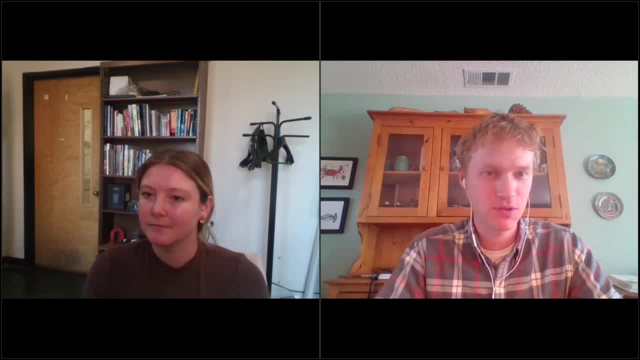 So maybe I'll start with some questions about dark earths, because they might not be familiar to everyone in the audience, So it might be interesting to do a little bit of a deep dive on them. Did dark earth soils exist anywhere besides the tropics? 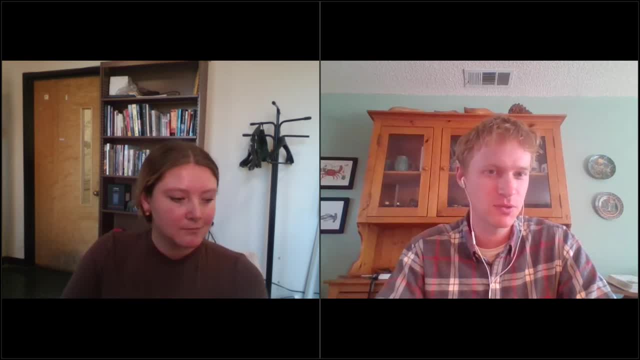 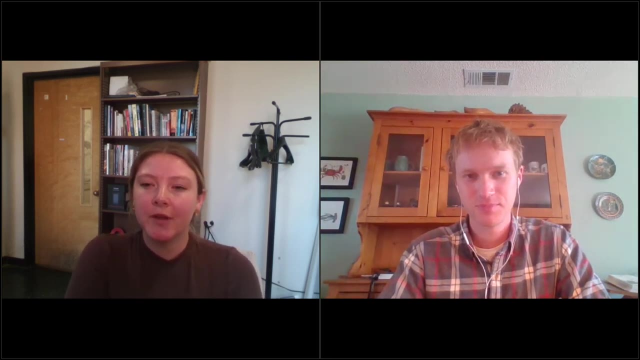 I mostly feel like I hear about them in the context of tropical soils, But what do you know about their geographic distribution globally? I think that's a really good question And what's exciting about dark earths? because they have only really recently been examined, right? 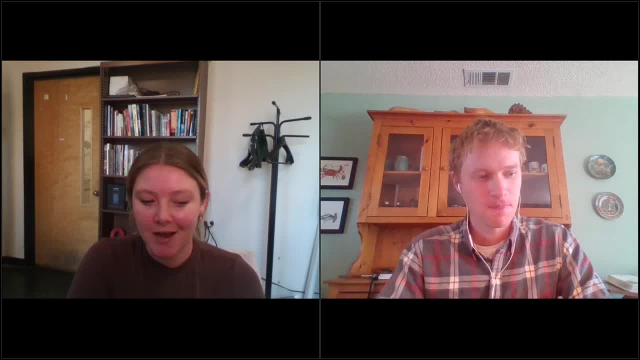 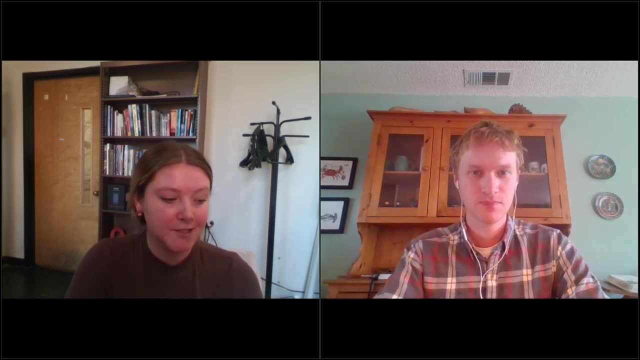 We've been working with soil since the beginning of agricultural development, But Western science has only been studying these dark earths since about the 90s, And there have been other soils that are considered dark earths in other parts of the world. There are some papers about soil out of the Czech Republic and other places. 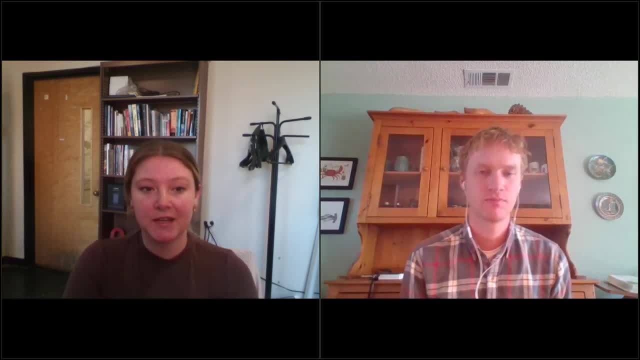 But for me I really do consider the dark earths that I'm talking about to be something more specifically related to indigenous knowledge and human activity. So there has been some questions sometimes about whether there are more natural processes that can contribute to these localized sites that have increased organic matter. 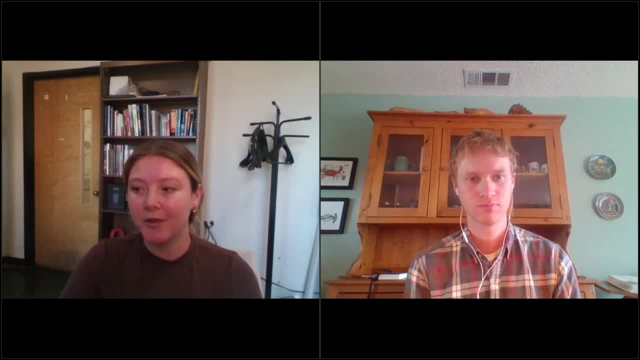 But more often than not, I believe that dark earths are characterized as such anthropogenic dark earths Because they have pottery remnants, other middens, and are not necessarily intentionally created, but definitely anthropogenic. So to answer that question, in short, I think that conversation is still ongoing. 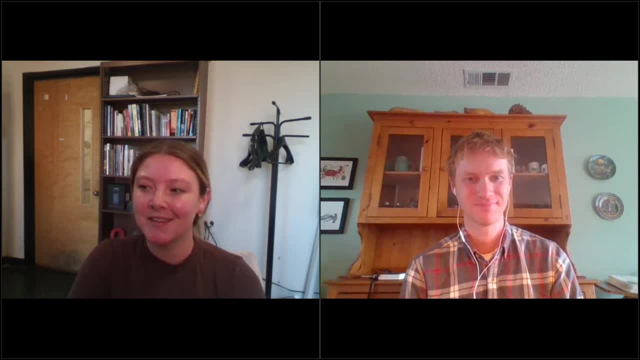 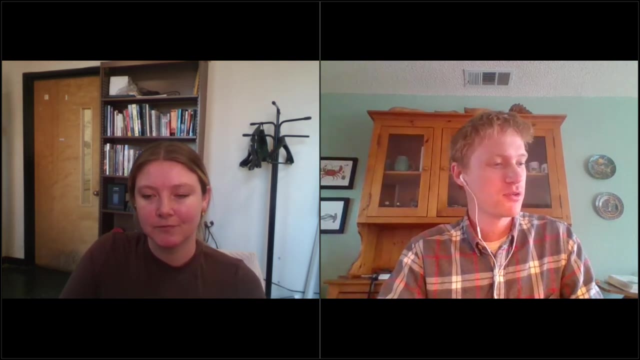 But from my perspective, there is a lot of relation to containing pyrogenic carbon, And I'm talking here. I'm talking here about anthropogenic dark earths. Okay, So to rip off another question that popped up in the chat here: 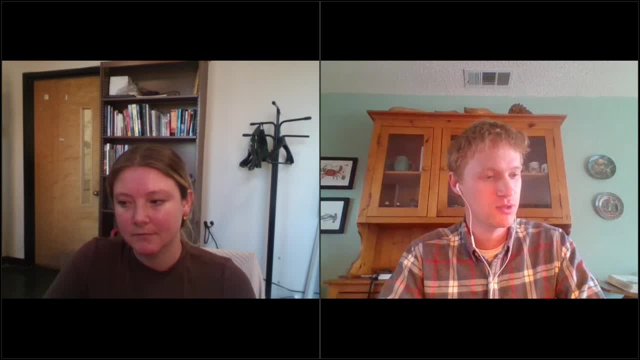 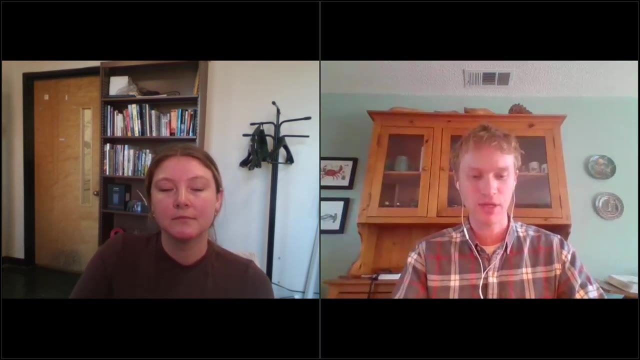 So it sounds like these particular soils require management, whether it's active or passive, Or they require humans to be importing organic matter from elsewhere. Is that your understanding that these soils are created by moving carbon From the landscape into one spot and concentrating it? 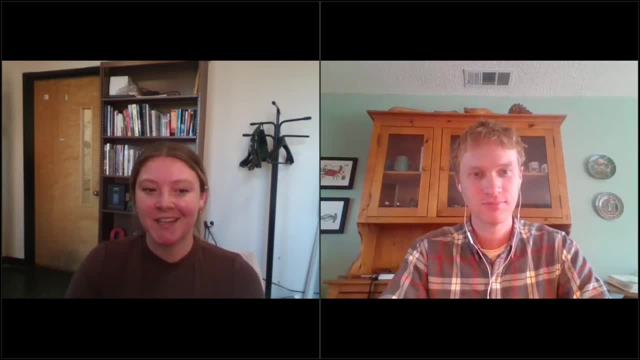 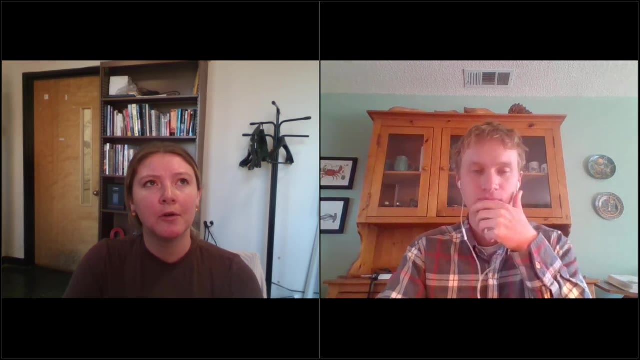 Yeah, So the first part of the question is very interesting. Land management and management of these dark earths is definitely a hot topic. But thinking about moving organic material from the landscape into the dark earths, I think that depends on what the land management was. 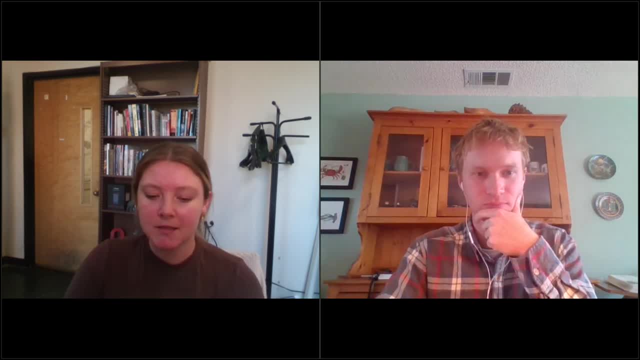 But I think the more common understanding is very localized household waste And so it depends on what you consider like relocation from out of the landscape. So it's very tied to agriculture and not just right like natural vegetation, If that answers your question. So we got a couple of questions about 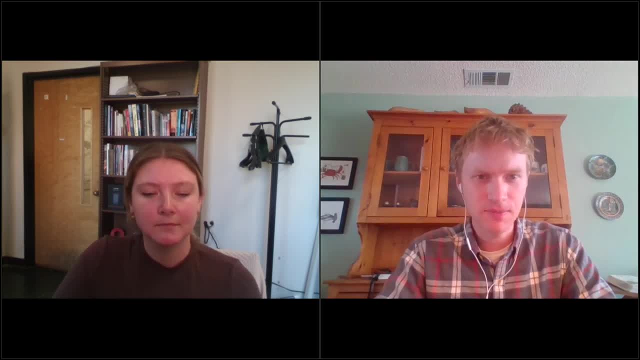 Time scales, And I know that this might require kinds of information that weren't in your particular study. But what do we know about how long it takes for a soil to approach these high levels of carbon? I mean, is there, are there insights from these tropical systems about you know, is it? 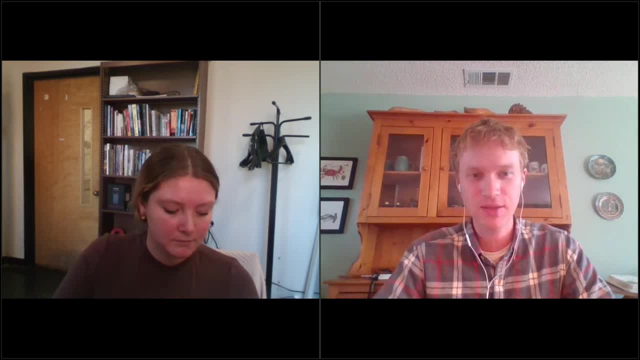 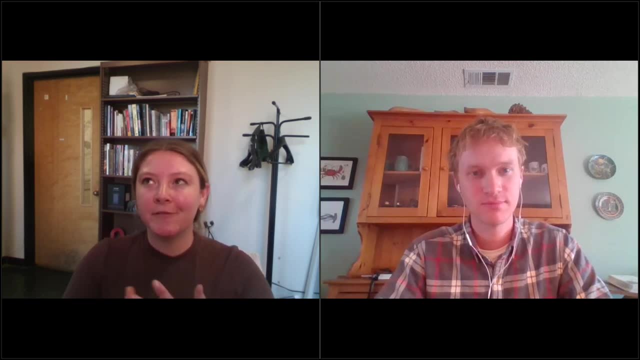 Is it a matter of decades or centuries or millennia of human influence? I really love that question because one of my favorite things about soil science is the different scales, And so I think to get that dark color so deep it does take time, So a lot of there are studies that have shown that these practices may have been going on for centuries, if not more than a thousand years. 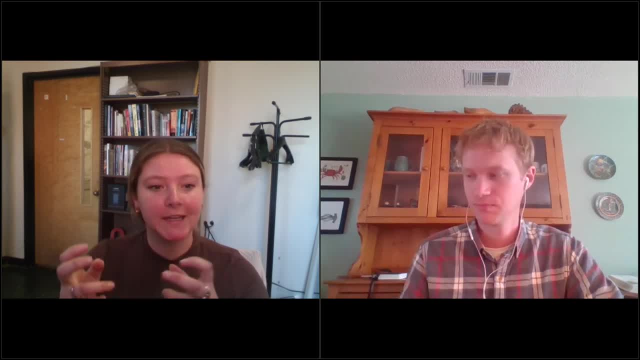 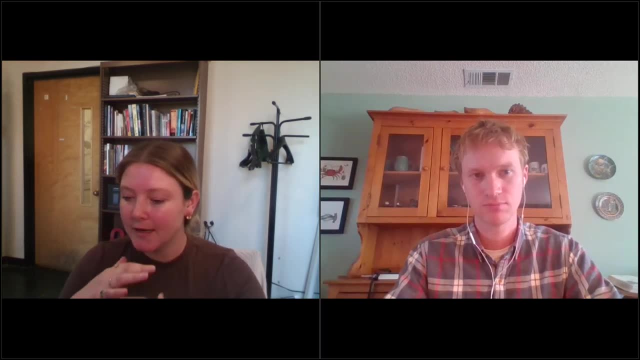 So, really. So you know, just thinking about This, Filling, so to speak, that soil profile could take quite a long time. But specifically, if you're looking at just a sample And thinking about the carbon content of that, That's where pyrogenic carbon can come in, because that can be energy dense, carbon dense and relatively stabilized. 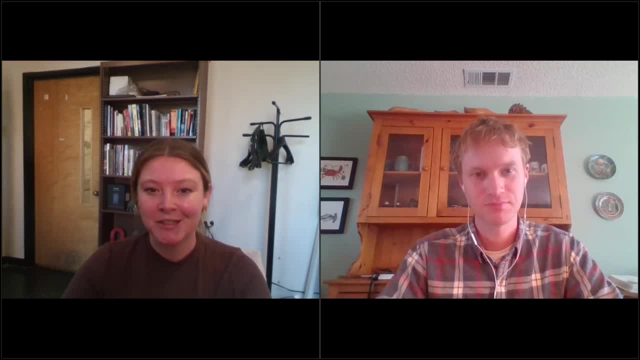 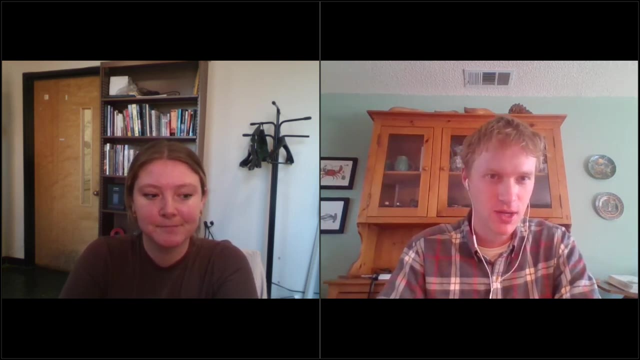 And that takes, you know, just within less than a year process right. So I think there's two different scales you're looking at when you're considering that question. So, about that pyrogenic carbon, I've got a question here from Bram Stone. 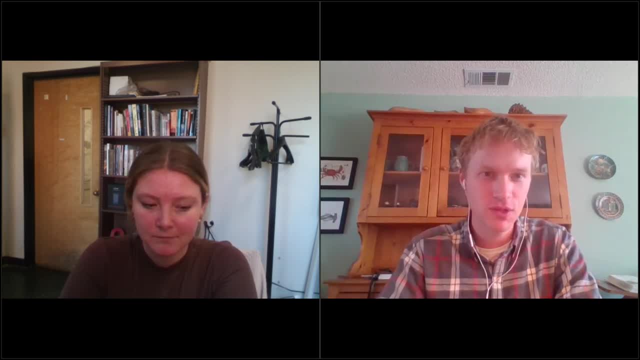 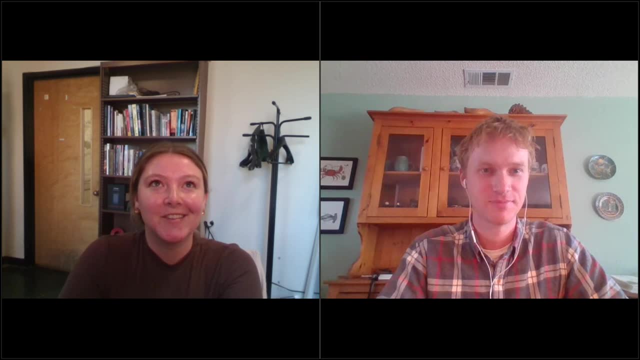 Does pyrogenic carbon offer a surface for carbon association analogous to mineral particles? That's a really good question that I'd like to look into. I do believe it provides a surface for organic matter association, but whether that's analogous to the soil mineral. 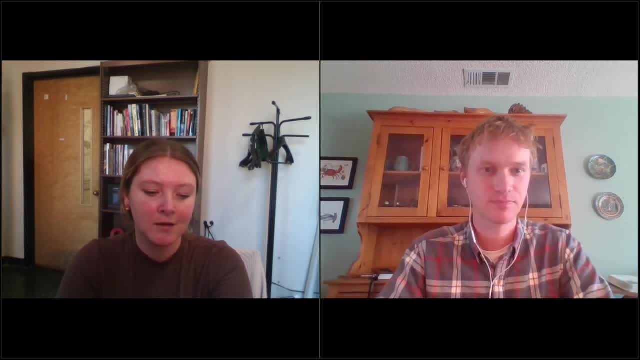 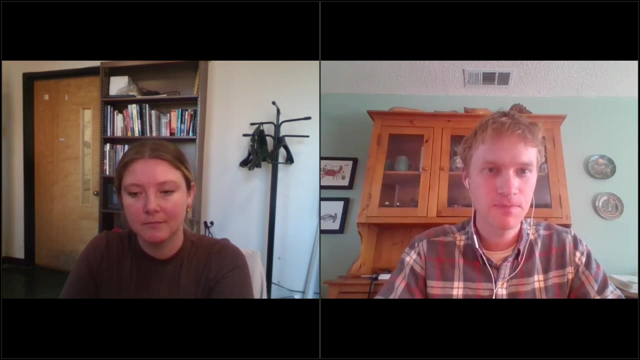 I'm not sure and most likely depends on the soil mineral in question. So but that's a good question. So another question here about the, the monolayer concept. So this question is: isn't Maher's monolayer equivalent limit of one? 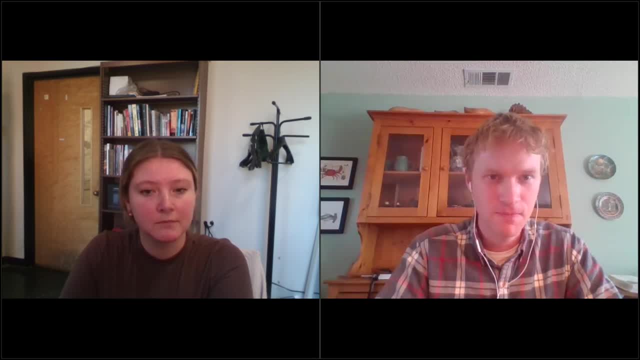 considering purely mineral associated organic matter, And so this question is then: in your measurements, isn't your EA data implicitly including particulate organic matter? So maybe this is sort of asking for a clarification about what your total carbon measurements were showing in those graphs. 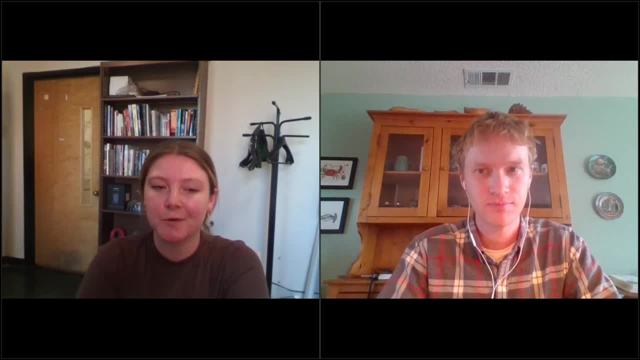 Yeah, so they were taken from bulk soil. That is correct. So I'll plug future talks or future papers. So that's what I've been working on over the past year and a half or so of my dissertation, performing those density separations and size separations. 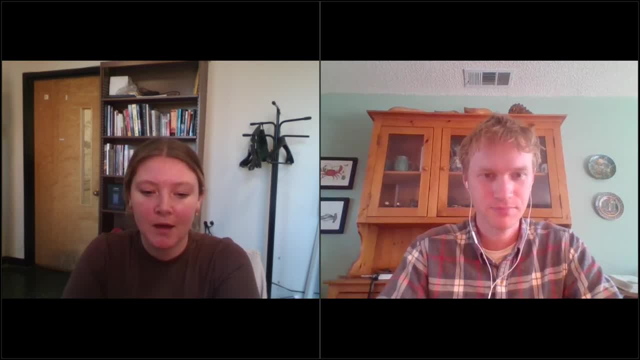 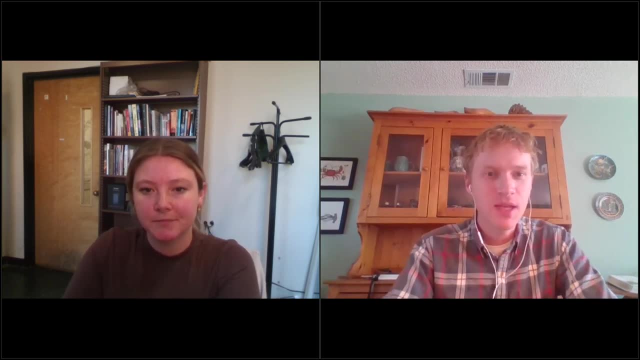 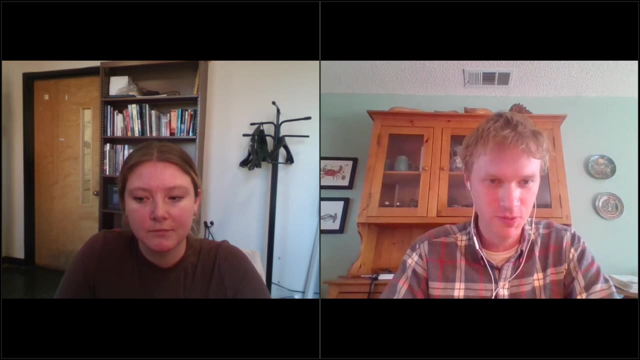 And then we'll be comparing the carbon concentrations to that as well. Yeah, it's a good question. And then there's another one in here, that's if I can paraphrase it. it's quite similar to one that was posed to Kat. but I'd like to hear your answer. How does aggregation play into this? I mean, the monolayer concept is based on surface area as the fundamental control, but if we think about minerals being organized into larger structures, how does that change? 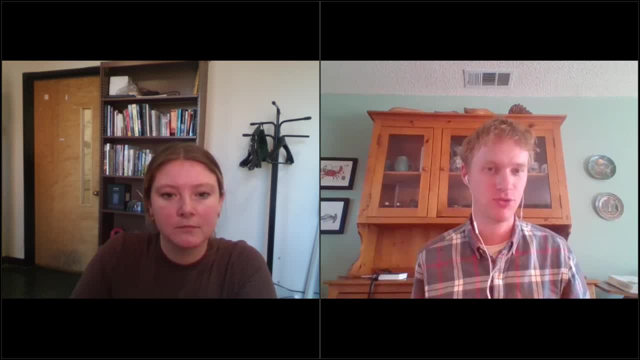 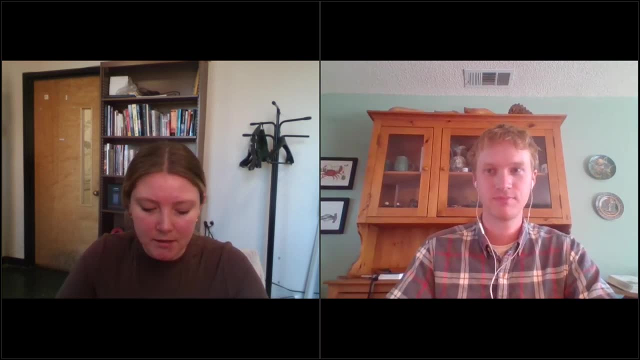 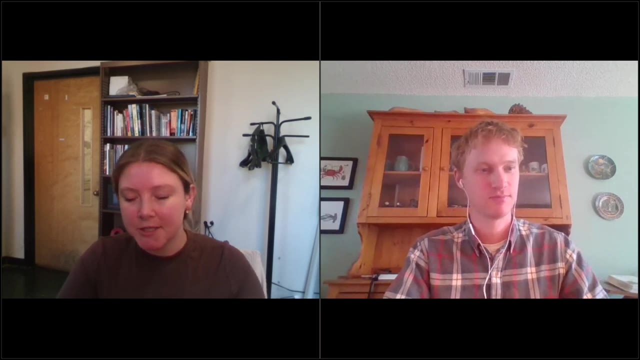 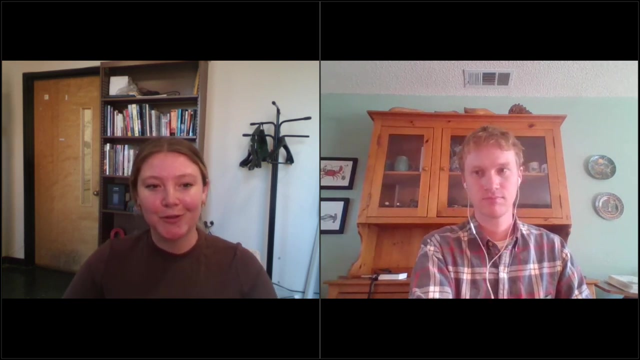 How does that change the way that we think about carbon saturation? Yeah, I actually think about this quite a bit, because soil carbon stabilization is different than soil carbon saturation, which I think we were Kat and I were alluding to with our talks. 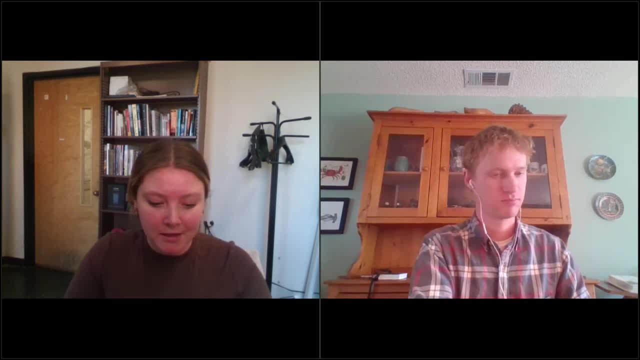 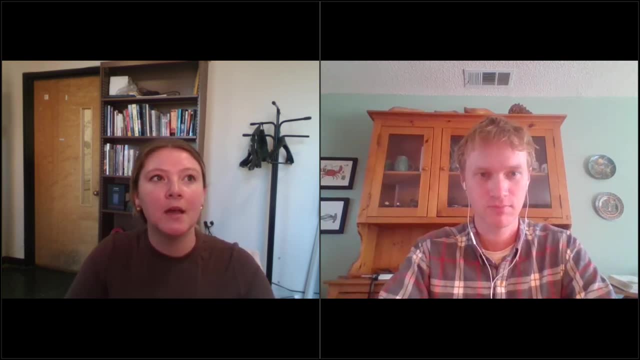 So soil or organic matter, soilQU�, organic carbon can be stabilized through our aggregation. that's, you know, definitely important, and having pyrogenic carbon and having char in the soil has been shown to increase aggregation. so not only is that maybe chemically persistent material, it can enhance further stabilization, but in 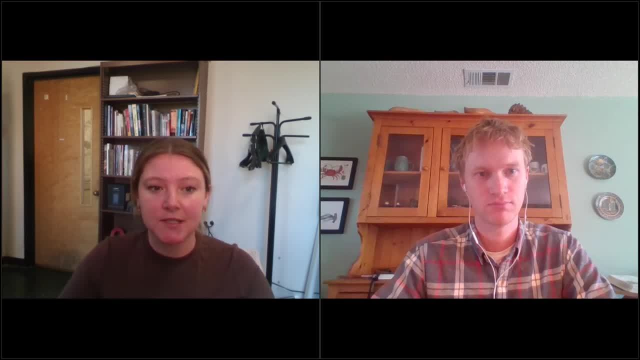 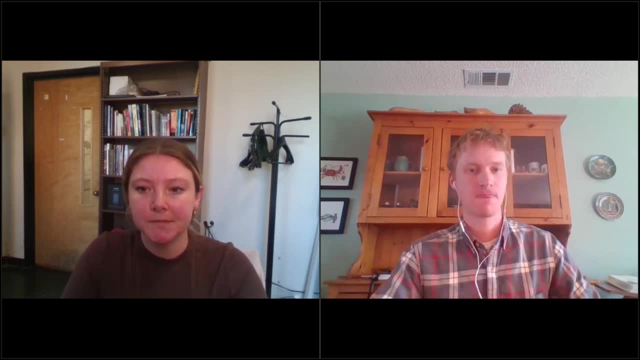 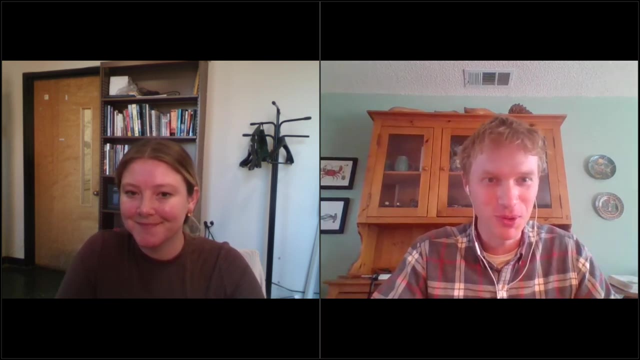 my opinion, the conversation about stabilization versus saturation can be tricky, and we have to be careful how we think about that. all right, well, there are so many questions to choose from at this point. oh, this one might be good to address. so this is about histosols. histosols still have an upper bound of 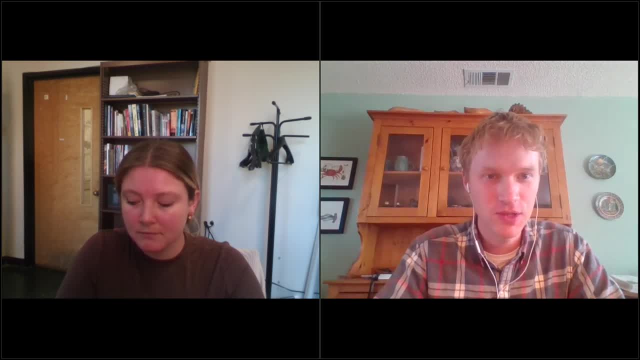 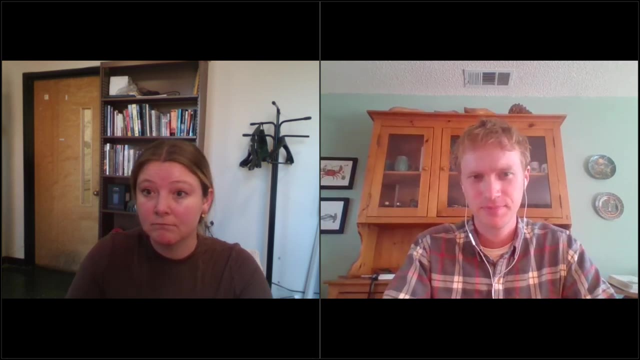 40 to 50 percent carbon. so what does this mean about the concept that there you know, there is no whole soil saturation? how do we think about wetland soils in this context? are they an exception, or do they fit into this framework? that's a good question. I don't know when I can punt to Kat as well, to give her. 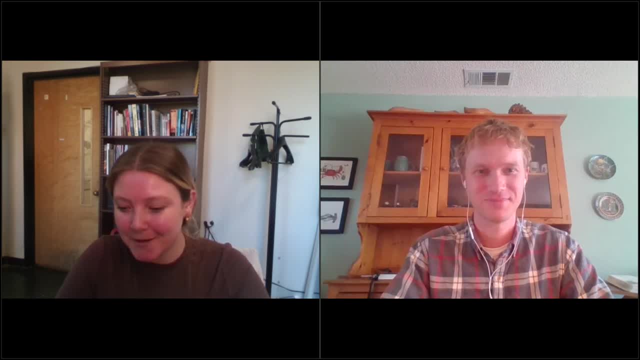 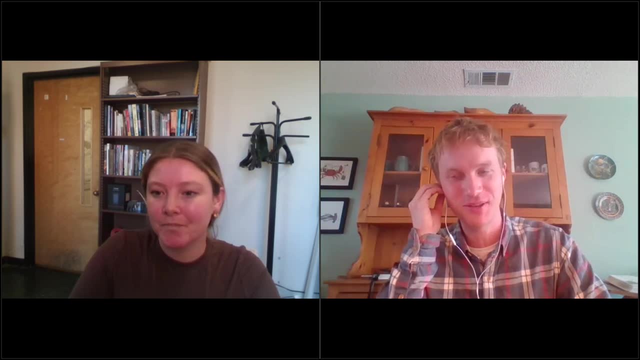 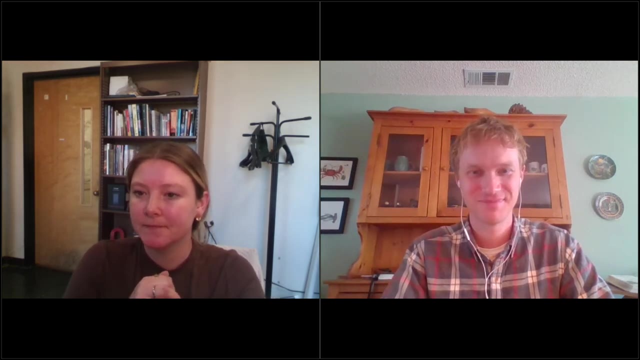 input. I definitely have to think about that, and that's a good question, Kat. if you're still on, feel free to chime in. maybe you've got a global scale perspective on this. yeah, I mean, I, I've. I, I do think about them differently personally, which is sort of why, in that particular organic matter, curve has a 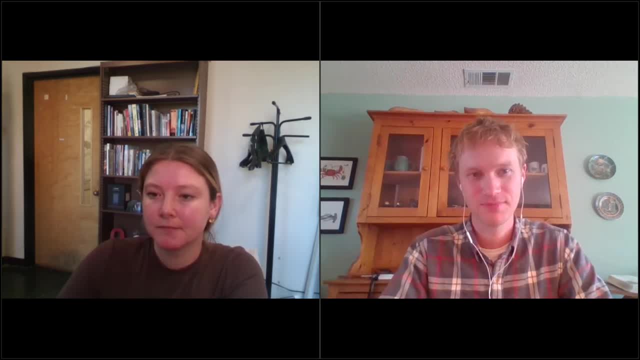 question mark at the end. you know there could be limits based on just sort of concentration and space constraints and depends on yeah, so I think there could be sort of limits, that I mean we see limits in sort of organic soils, but that's I don't know. I think of that very differently. I. tend to think more about the mineralogical limits in mineral soils. but yeah, I mean, certainly you could accrue, in theory, more particulate organic matter under the right conditions, up to much higher levels. and so yeah, I don't know if that answers the question more, if you want to add.